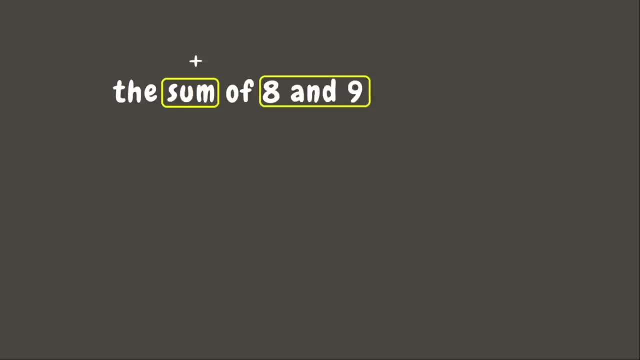 This means that we need to add 8 and 9.. So that is 8 plus 9.. And this is an example of a numerical expression. Next one: we have the sum of 4 and a number Again. our keyword here is sum, which means addition. 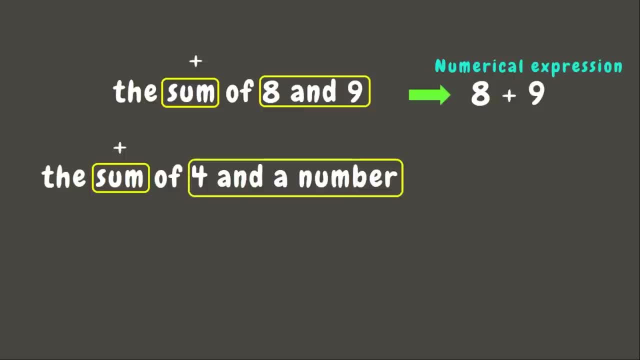 This means that we need to add 4 and a number Here. we do not know the value of a number, Therefore we are going to represent it by a letter. Let's say letter N. So that is 4 plus N. 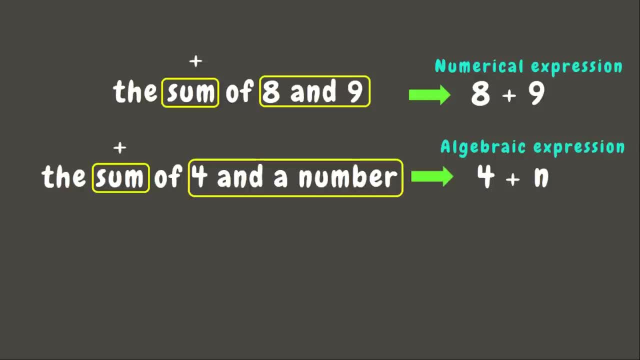 This is an example of algebraic expression. Next one: we have the sum of 4 and a number is 7.. Again, our keyword here is the word sum, which means addition, And we need to add 4 and a number which is 4 plus N. 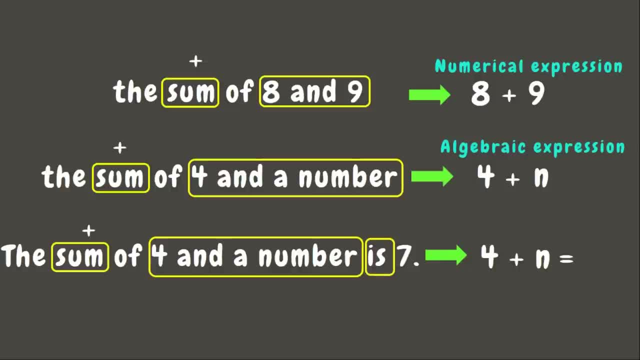 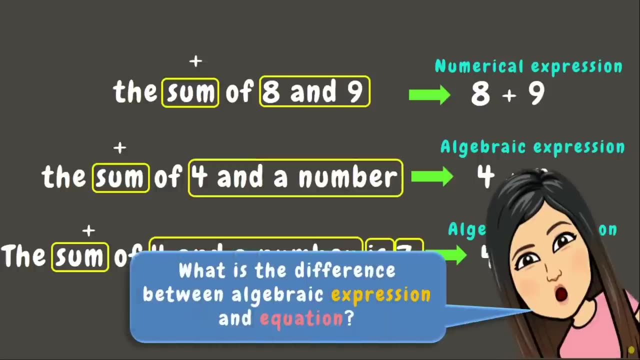 And the word is represents equal sign. Therefore, 4 plus N is equal 7.. This is an example of algebraic equation. Now do you know what is the difference between algebraic expression and equation? Let's go and take a look. 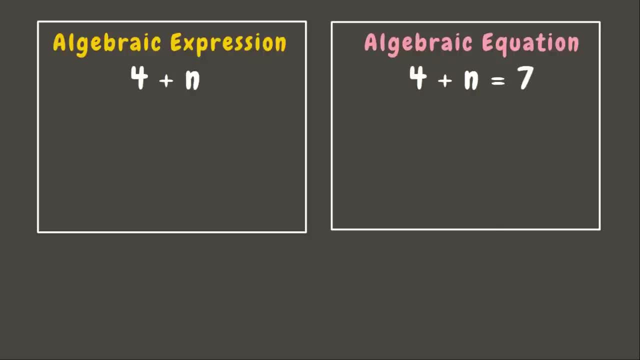 Let us discuss the differences between expression and equation. In algebraic expression, it is a mathematical phrase. For example, we have the sum of 4 and a number And, as we can see, this is not a complete sentence, While the algebraic equation is a mathematical sentence. 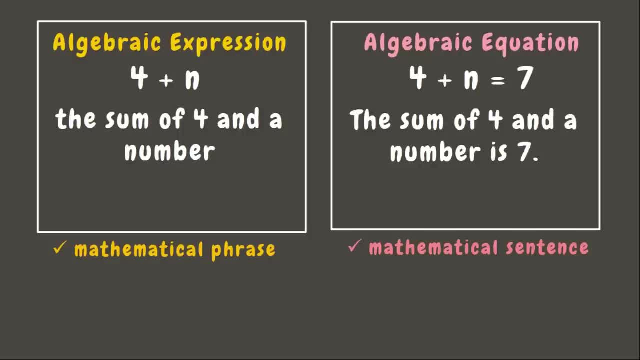 For example, we have the sum of 4 and a number is 7.. Another one is: algebraic expression has no equal sign, While in algebraic equation it has equal sign which, represented by the word, is Lastly in an expression. 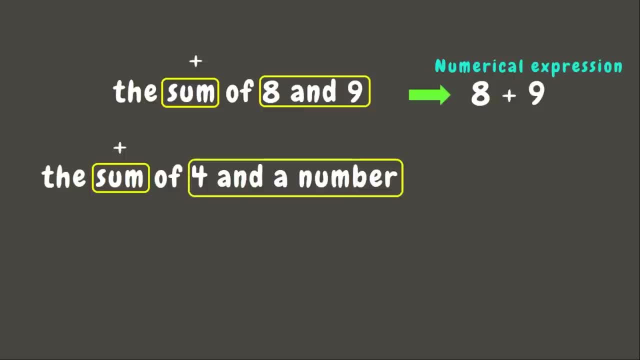 This means that we need to add 4 and a number Here. we do not know the value of a number, Therefore we are going to represent it by a letter. Let's say letter N. So that is 4 plus N. 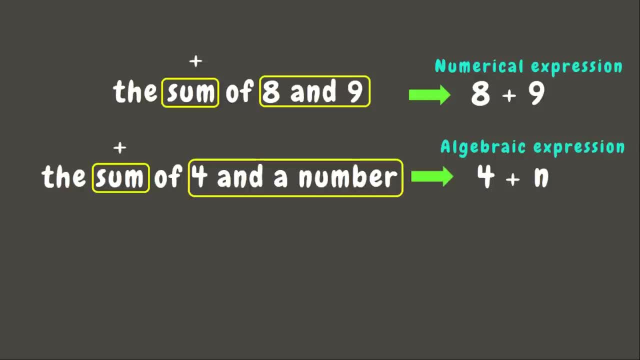 This is an example of algebraic expression. Next one: we have the sum of 4 and a number is 7.. Again, our keyword here is the word sum, which means addition, And we need to add 4 and a number which is 4 plus N. 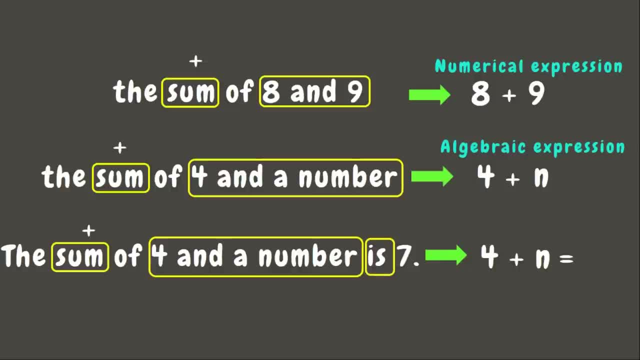 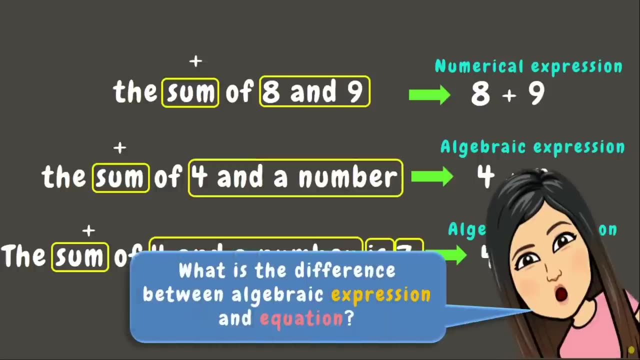 And the word is represents equal sign. Therefore, 4 plus N is equal 7.. This is an example of algebraic equation. Now do you know what is the difference between algebraic expression and equation? Let's go and take a look. 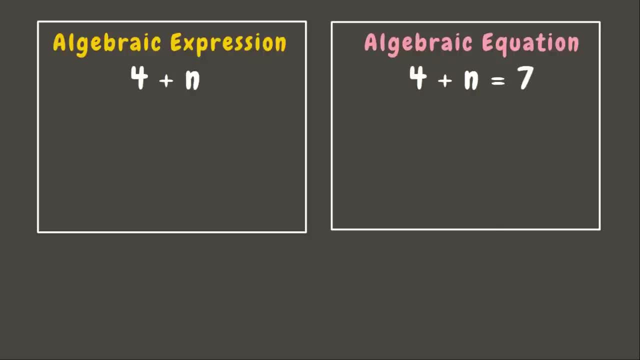 Let us discuss the differences between expression and equation. In algebraic expression, it is a mathematical phrase. For example, we have the sum of 4 and a number And, as we can see, this is not a complete sentence, While the algebraic equation is a mathematical sentence. 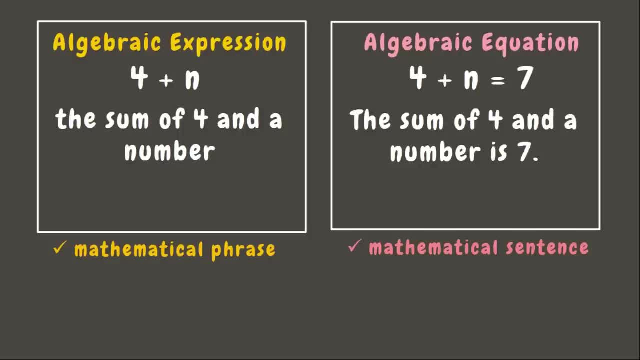 For example, we have the sum of 4 and a number is 7.. Another one is: algebraic expression has no equal sign, While in algebraic equation it has equal sign which, represented by the word, is Lastly in an expression. 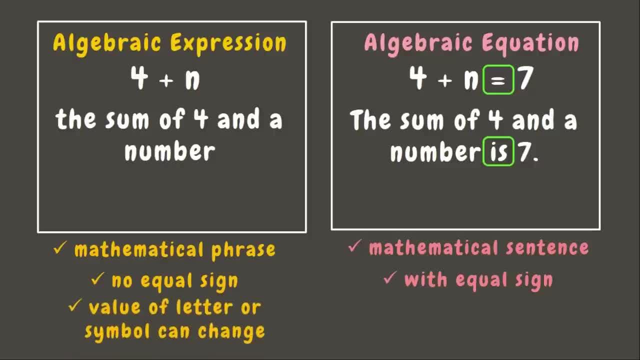 a value of the letter or the symbol can change. For example, here we have 4 plus N. We can say that the value of N is 5.. So that would be 4 plus 5.. Or we can say that the value of N here is 9.. 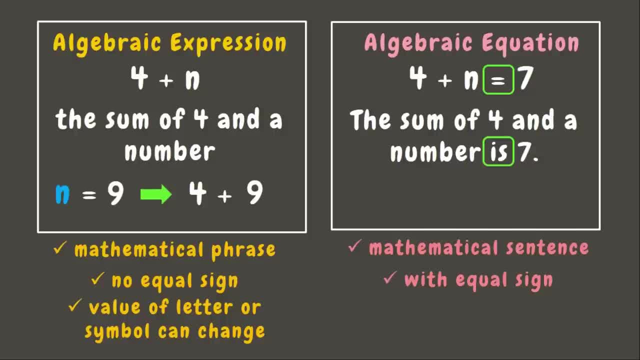 So that would be 4 plus 9.. Or let us say it is equal 2.. So that would be 4 plus 2.. On the other hand, in algebraic equation the value of the letter or the symbol cannot be changed. 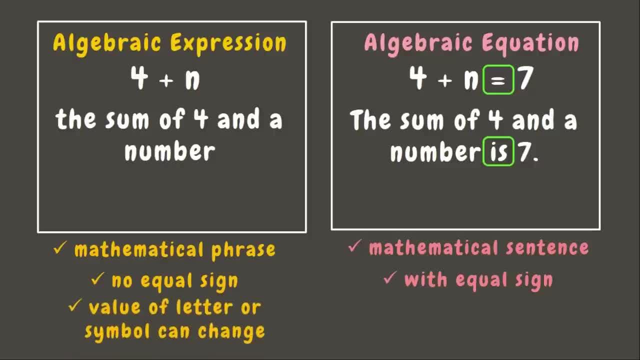 a value of the letter or the symbol can change. For example, here we have 4 plus N. We can say that the value of N is 5.. So that would be 4 plus 5.. Or we can say that the value of N here is 9.. 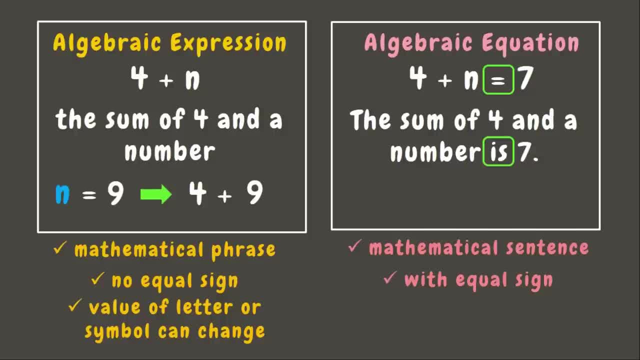 So that would be 4 plus 9.. Or let us say it is equal 2.. So that would be 4 plus 2.. On the other hand, in algebraic equation the value of the letter or the symbol cannot be changed. 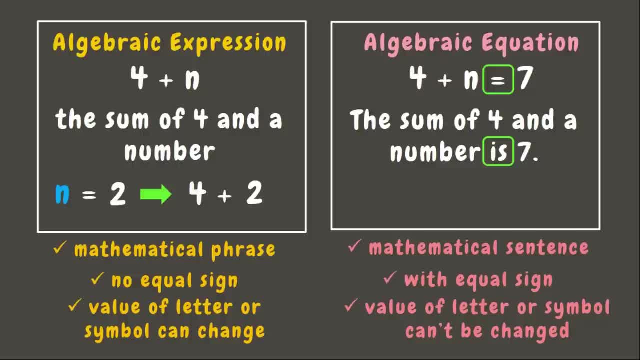 It has a fixed value or fixed answer Here. in 4 plus N equals 7, we cannot say that the value of N is 9.. As it will not say that the equation is correct If we say that the value of N here is 9,. 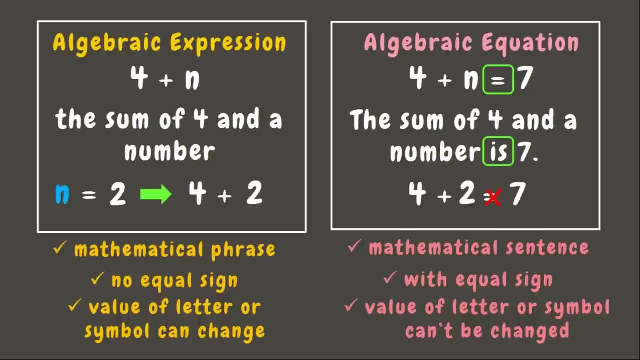 and the value of N here is 2, the equation would be wrong. What if we say that the value of N here is 3? 4 plus 3 equals 7. And that is the correct value of N. Wonderful, Now that you know the differences. 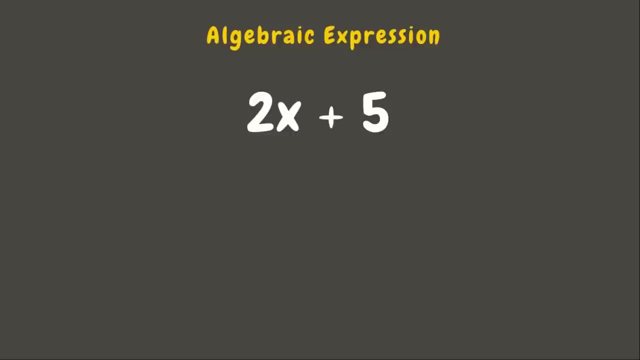 let us move on to the parts of algebraic expression. The first one is the variable. The variable is any letter or symbol that represents a number. Here the variable is letter x. The next one is the coefficient. The coefficient is the constant value used with the variable. 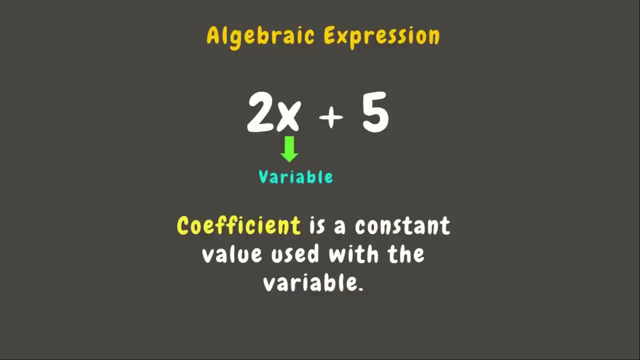 It is the factor or the number being multiplied to a variable. Here the coefficient is 2.. We can always find the coefficient before the variable. The next one is the constant. The constant is a fixed value that does not change. Here the constant is number 5.. 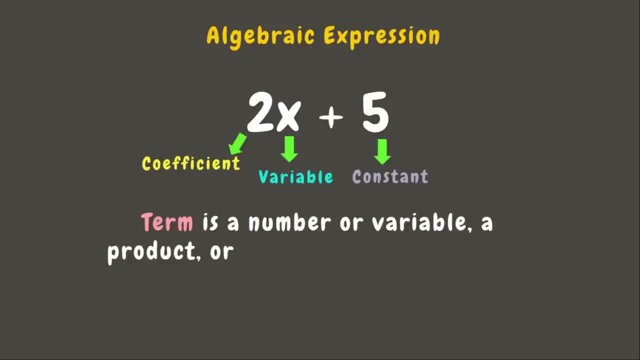 And lastly, we have the term. The term is a number or variable, a product or quotient of a number and variable separated by plus or minus sign. Here, in a given example, we have the plus sign And it separates two terms. 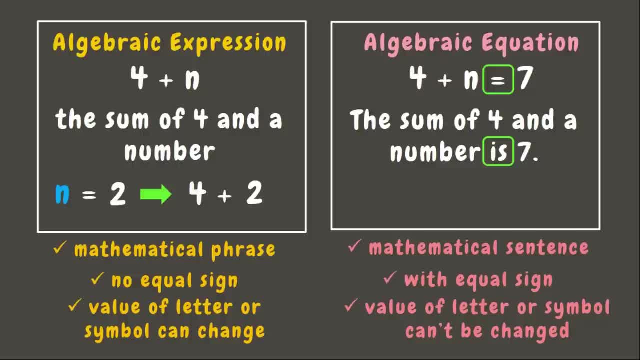 It has a fixed value or fixed answer Here. in 4 plus N equals 7, we cannot say that the value of N is 9.. As it will not say that the equation is correct If we say that the value of N here is 9,. 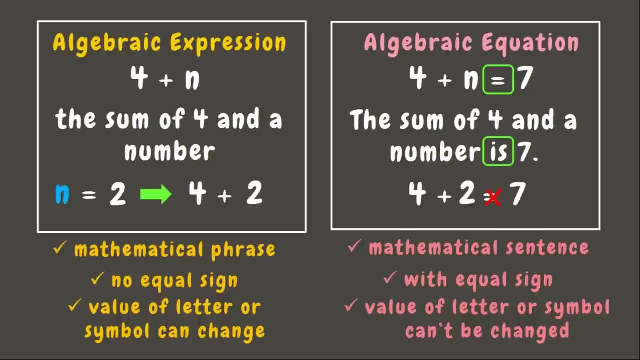 and the value of N here is 2, the equation would be wrong. What if we say that the value of N here is 3? 4 plus 3 equals 7. And that is the correct value of N. Wonderful, Now that you know the differences. 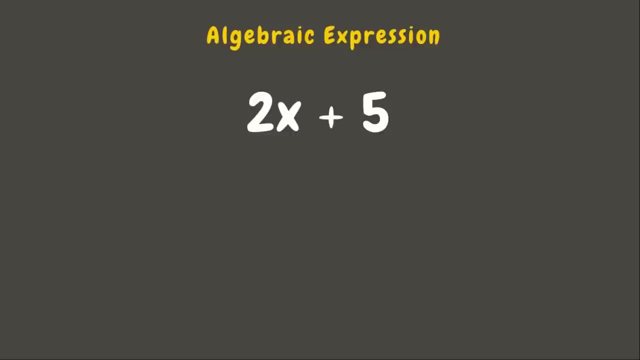 let us move on to the parts of algebraic expression. The first one is the variable. The variable is any letter or symbol that represents a number. Here the variable is letter x. The next one is the coefficient. The coefficient is the constant value used with the variable. 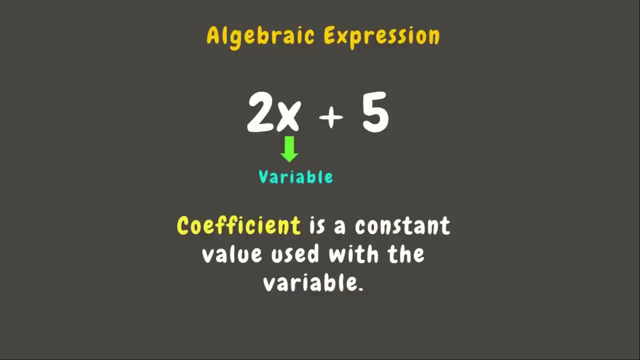 It is the factor or the number being multiplied to a variable. Here the coefficient is 2.. We can always find the coefficient before the variable. The next one is the constant. The constant is a fixed value that does not change. Here the constant is number 5.. 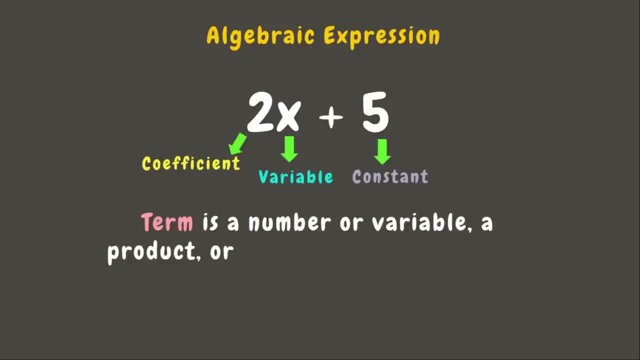 And lastly, we have the term. The term is a number or variable, a product or quotient of a number and variable separated by plus or minus sign. Here, in a given example, we have the plus sign And it separates two terms. 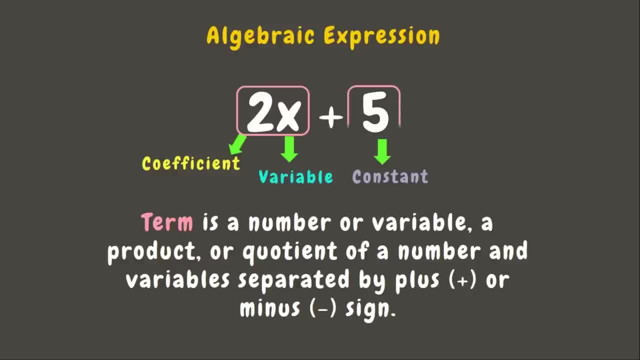 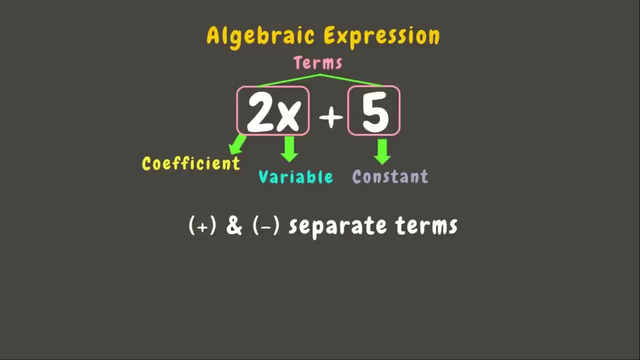 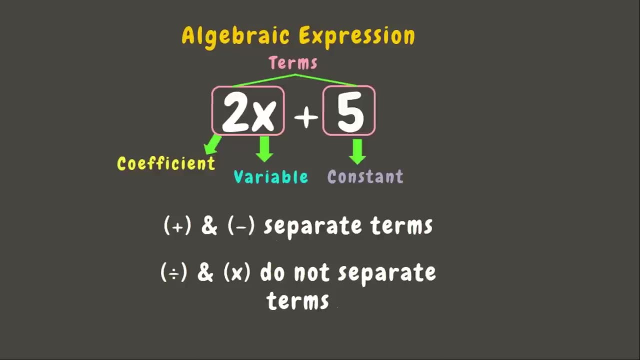 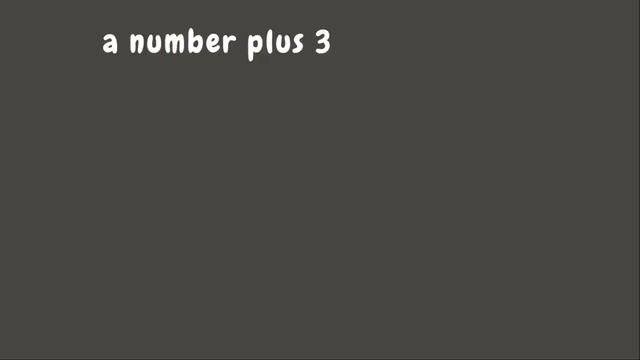 which are 2x and 5.. Remember that addition and subtraction only separate terms, while division and multiplication do not separate terms. Now that you already know the parts and the differences between equation and expression, let us go and translate some verbal expressions. 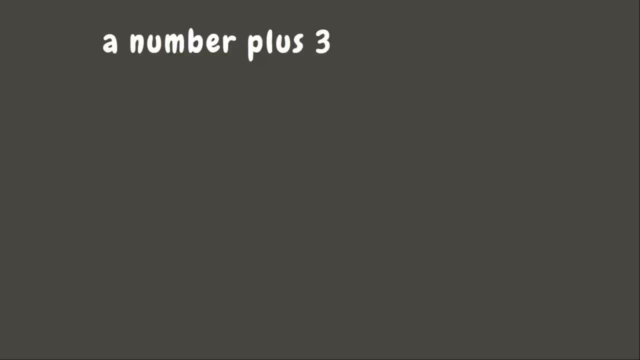 Here we have a number plus 3.. First one that you need to know is: what is the missing here? The missing here is a number. This means that we are going to represent it by a variable, any letter that we would like to. 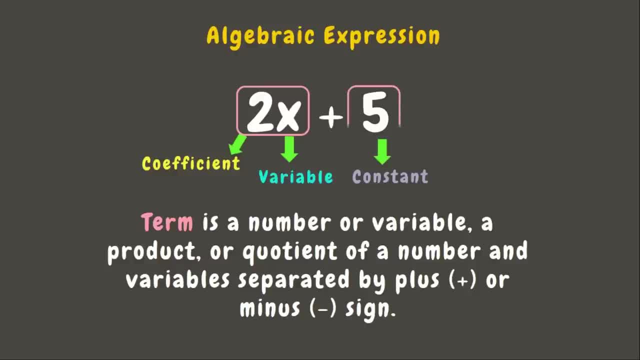 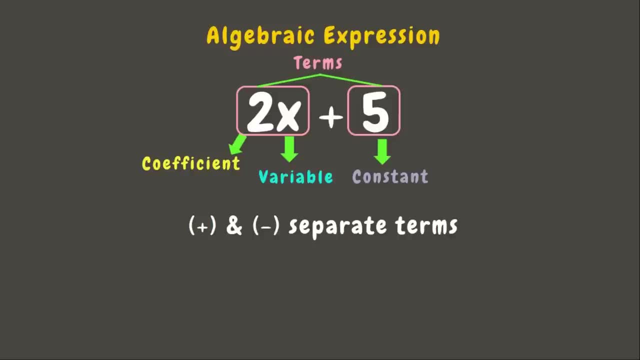 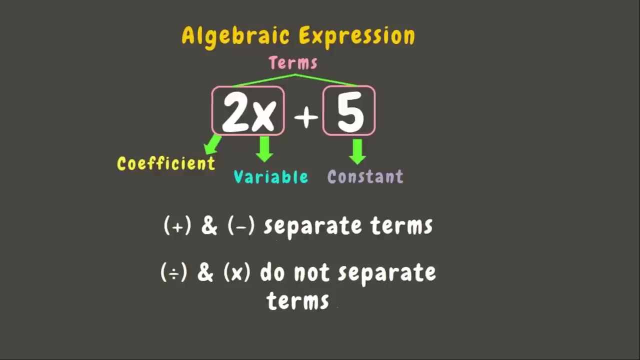 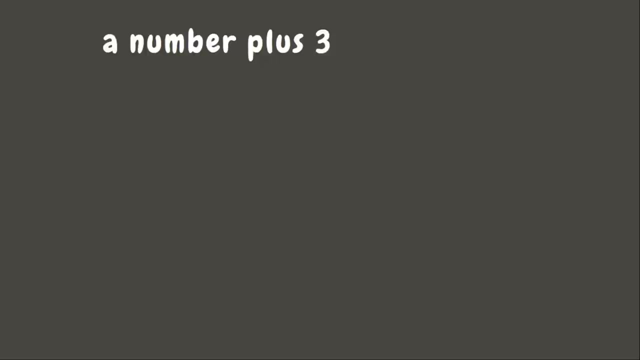 which are 2x and 5.. Remember that addition and subtraction only separate terms, while division and multiplication do not separate terms. Now that you already know the parts and the differences between equation and expression, let us go and translate some verbatim. 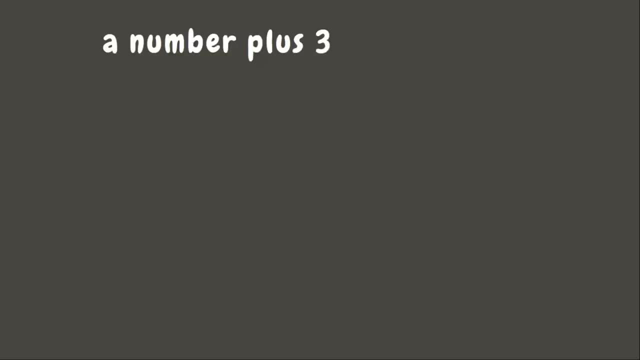 Here we have a number plus 3.. The first one that you need to know is: what is the missing here? The missing here is a number. This means that we are going to represent it by a variable, any letter that we would like to. 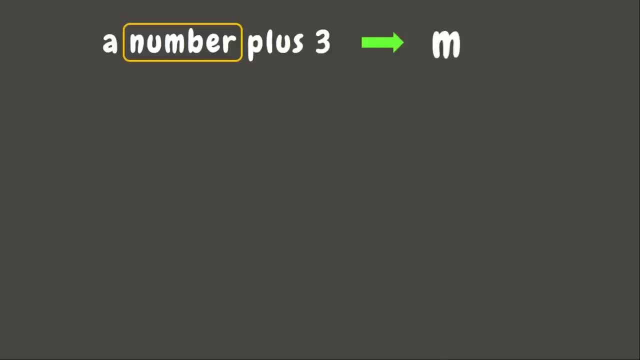 Let's say I want letter M. The next keyword here would be the word plus, which means addition. So that is M M plus 3. So our algebraic expression here is M plus 3.. Now let's have another example. 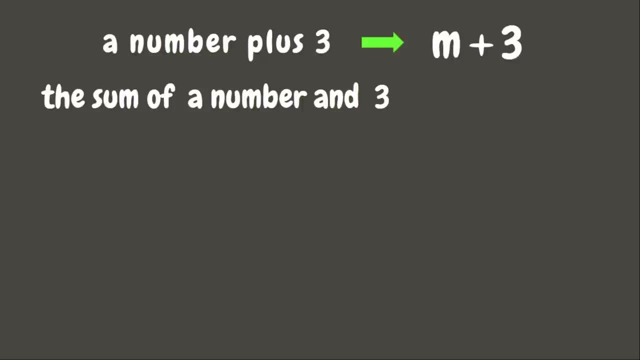 We have the sum of a number and 3.. Again, let's take a look for some keywords Here. the keywords that we have is the word sum, which means addition. Therefore, we need to add a number which can be represented by a variable. 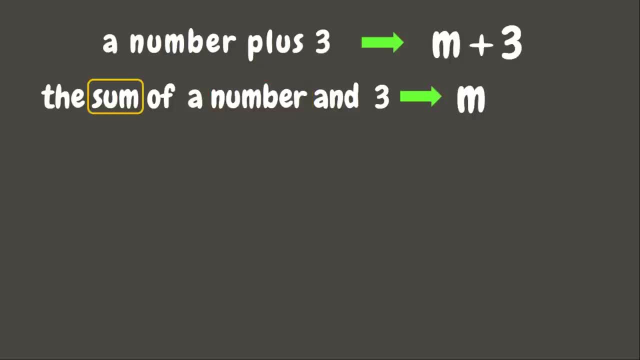 let's say letter M and the number 3. So that is M plus 3.. Very good, Let's have another one. We have M increased by 3. Here we already have a variable which is M, So let us write M. 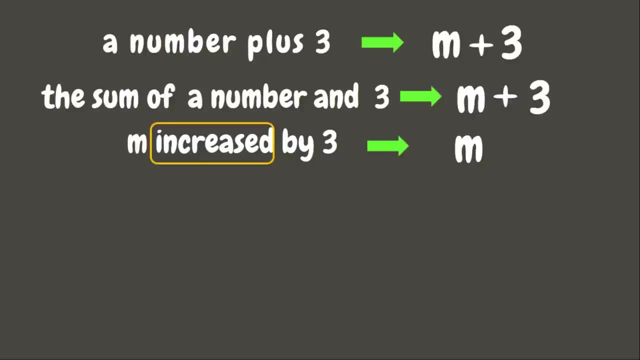 Next we have the keyword increased by. Increased by represents addition, So that would be a plus sign. And lastly, the number 3.. Next one, we have 3 added to M. So again we already have a variable which is M. 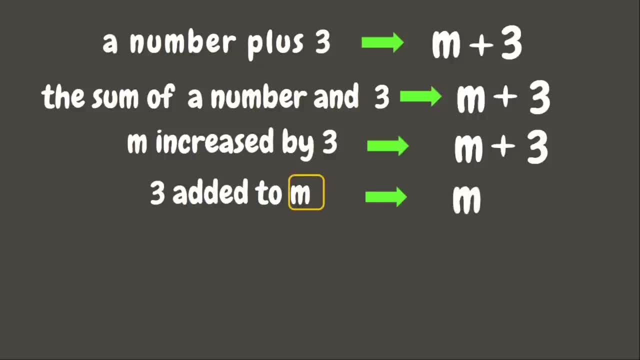 And we need to add 3 to it. So that is M plus 3.. Next one: we have 3 more than M. Again, our variable here is M And the word more than represents addition, And we have 3.. 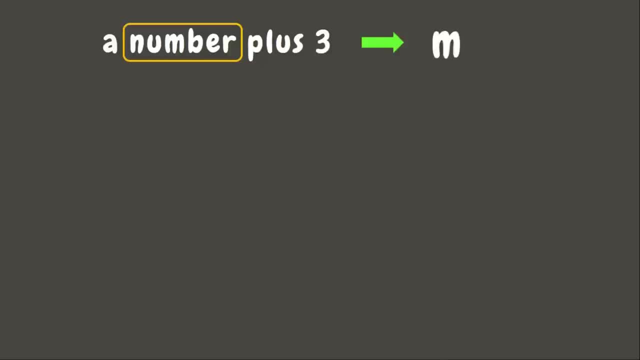 Let's say I want letter M. The next keyword here would be the word plus, which means addition. So that is M plus 3.. So our algebraic expression here is M plus 3.. Now let's have another example. We have the sum of a number and 3.. 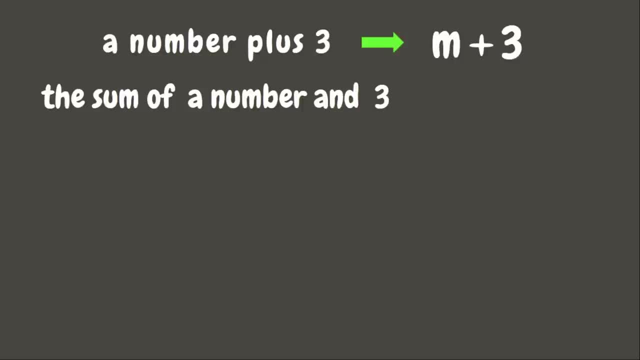 Again, let's take a look for some keywords Here. the keywords that we have is the word sum, which means addition. Therefore, we need to add a number which can be represented by a variable, let's say letter M and the number 3.. 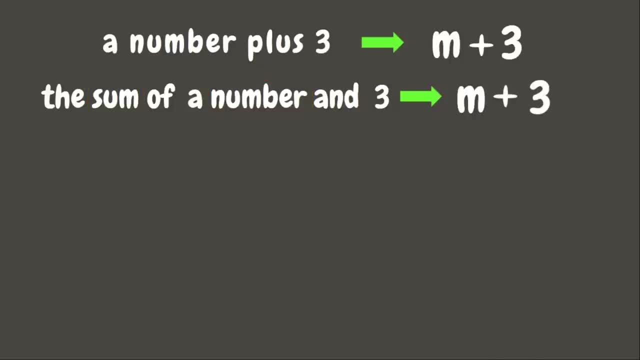 So that is M plus 3.. Very good, Let's have another one. We have M increased by 3.. Here we already have a variable which is M, So let us write M. Next we have the keyword increased by Increased by represents. 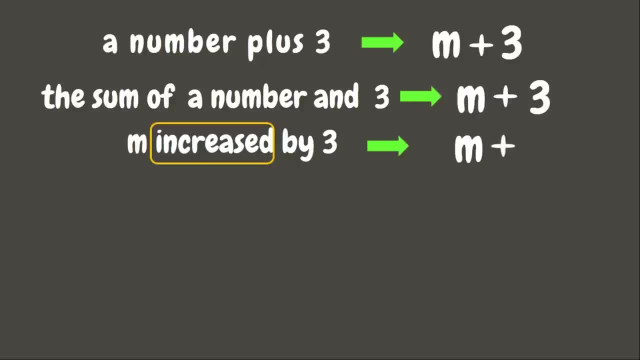 addition, So that would be a plus sign. And lastly, the number 3.. Next one: we have 3 added to M. So again, we already have a variable which is M And we need to add 3 to it. 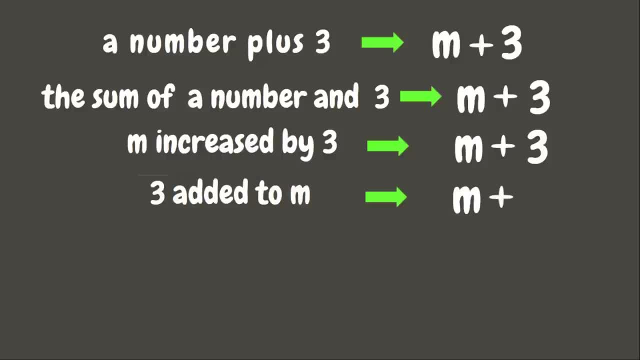 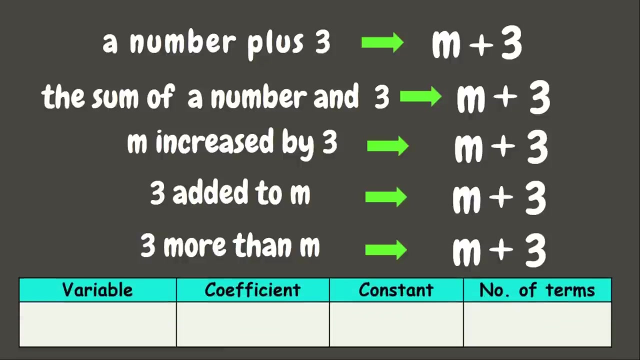 So that is M plus 3.. Next one: we have 3 more than M. Again, our variable here is M And the word more than represents addition, And we have 3.. So that is M plus 3.. Now let us identify which are the variable. 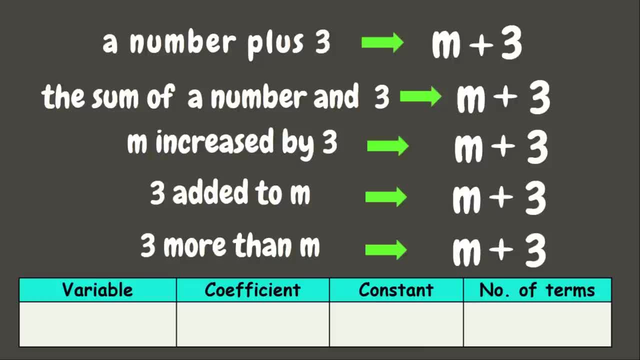 coefficient, constant and the number of terms here in our given algebraic expression, The variable here is the letter, which is M. Very good, Next one. let us take a look for the coefficient. Again, the coefficient is the number that we see before the variable. 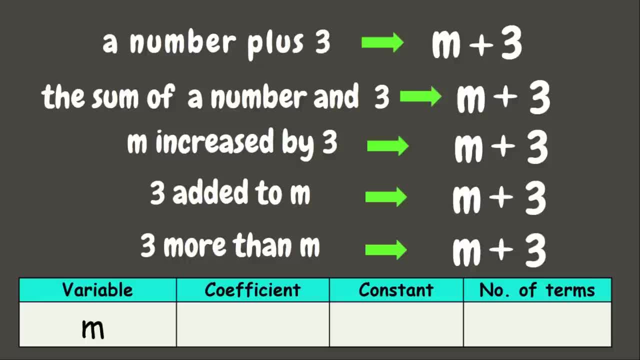 As we can see, there is no number before a variable here, But it doesn't mean that we do not have a coefficient. Remember that a coefficient is a factor or a number multiplied to a variable, All variables that do not have a number beforehand. 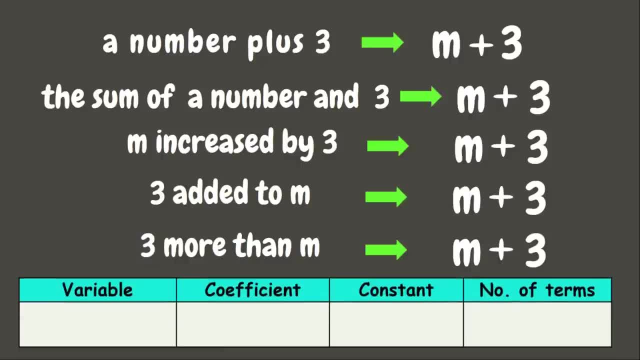 So that is M plus 3.. Now let us identify which are the variable, coefficient, constant and the number of terms here in our given algebraic expression. The variable here is the letter, which is M. Very good, Next one, let us take a look. 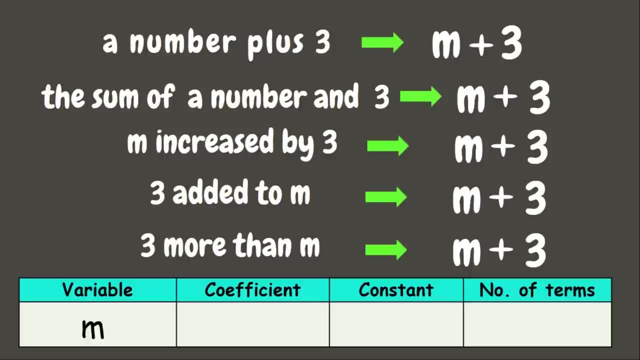 for the coefficient. Again, the coefficient is the number that we see before the variable. As we can see, there is no number before a variable here, But it doesn't mean that we do not have a coefficient. Remember that a coefficient is a factor or a number. 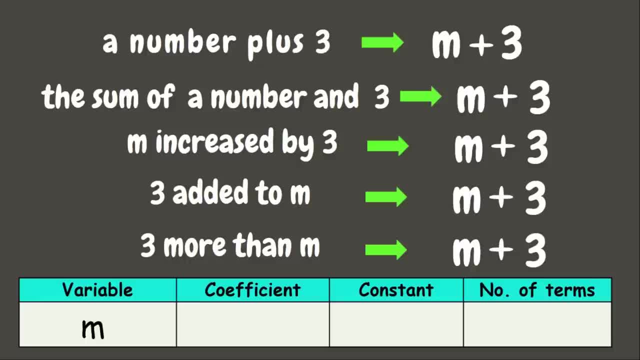 multiplied to a variable- All variables that do not have a number beforehand- has a coefficient of 1. Because it means 1 times M, which is equals M. So the coefficient here is 1.. Next one: the constant here is Very good. 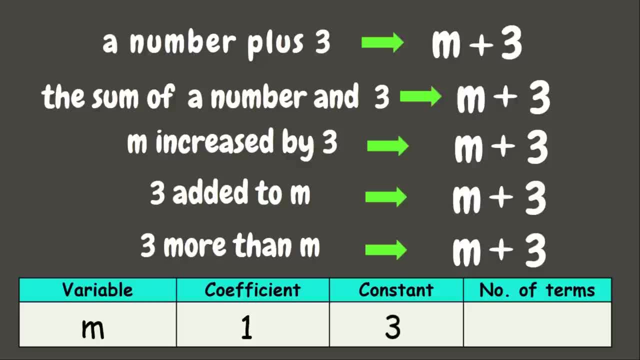 It is 3.. And let us count the number of terms. Since this algebraic expression is separated by a plus sign for addition, our terms here are M and 3. So we have 2 terms. Great job. Let's have another example. 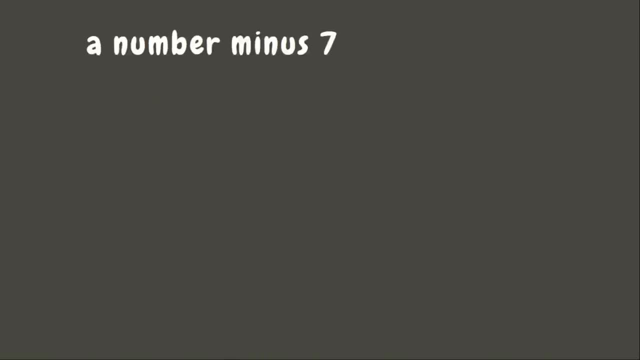 Next one: we have a number minus 7.. Again, we have here a number which can be represented by a variable. So let us say letter F. Our next keyword here is the word minus, which represents subtraction, And there is 7.. 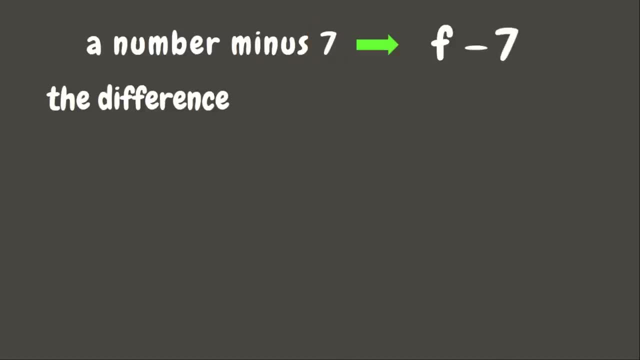 So that is F minus 7.. Next one: we have the difference of F and 7. So again, let us take a look for some keywords. We have difference And the difference represents subtraction, So we need to subtract F and 7.. 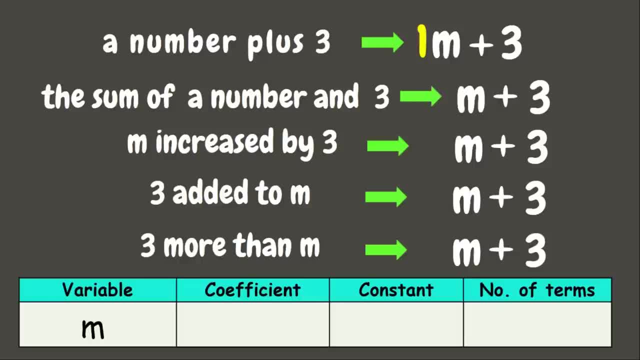 has a coefficient of 1. Because it means 1 times M, which is equals M. So the coefficient here is 1.. Next one: the constant here is Very good, It is 3.. And let us count the number of terms. 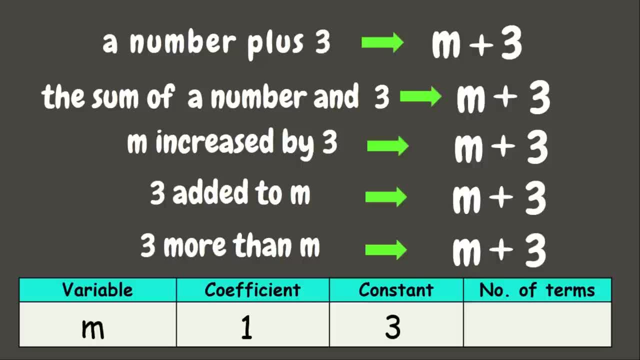 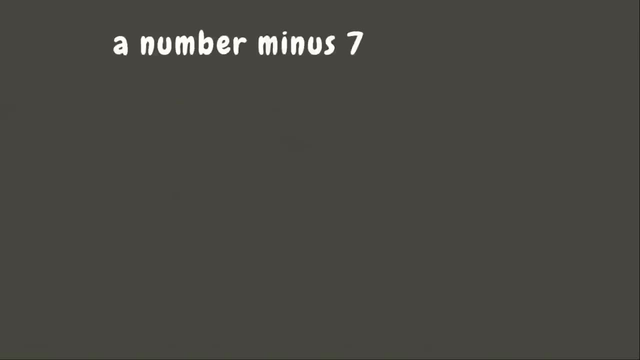 Since this algebraic expression is separated by a plus sign for addition, our terms here are M and 3. So we have 2 terms. Great job, Let's have another example. Next one: we have a number minus 7.. Again, we have here a number. 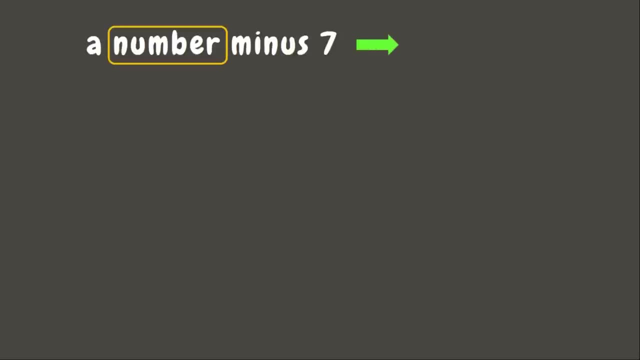 which can be represented by a variable. So let us say letter F. Our next keyword here is the word minus, which represents subtraction, And there is 7. So that is F minus 7.. Next one: we have the difference of F and 7.. 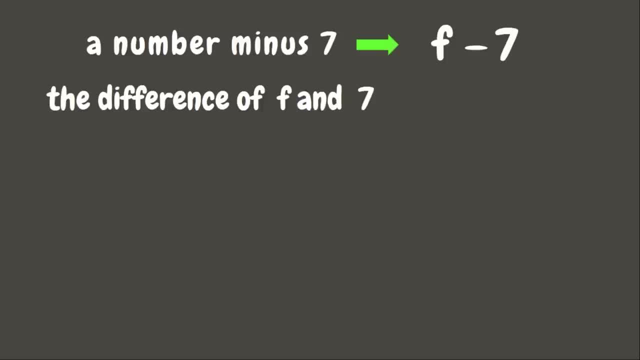 So again, let us take a look for some keywords. We have difference And the difference represents subtraction, So we need to subtract F and 7.. All right, Let us have another example. We have F decreased by 7. So our variable here is F. 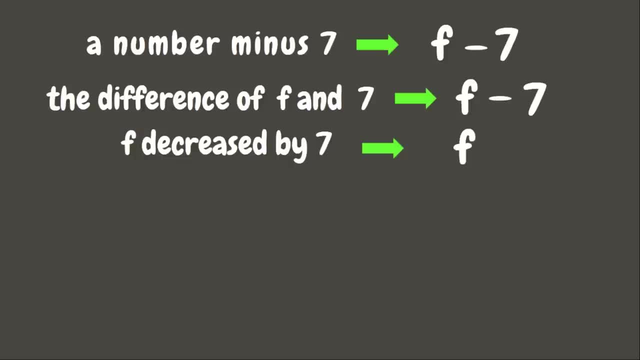 And we need to decrease this one, which represents subtraction, by 7.. Next example: we have 7 subtracted from F, So our variable here is the letter F And we need to subtract 7 from it, So that will be F minus 7.. 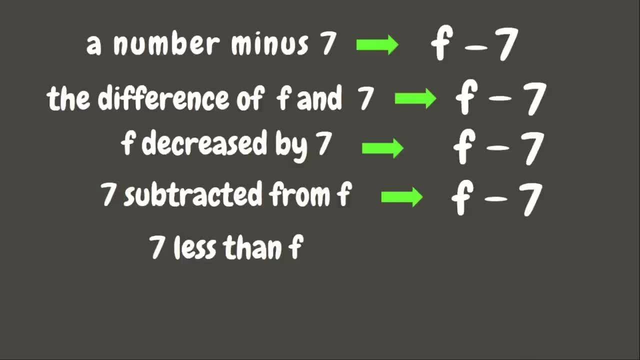 And lastly, we have 7 less than F And our variable again here is letter F And our keyword is less than, which means subtraction 7.. So that is F minus 7.. Now let us identify the variable. here, Again, our variable is the letter. 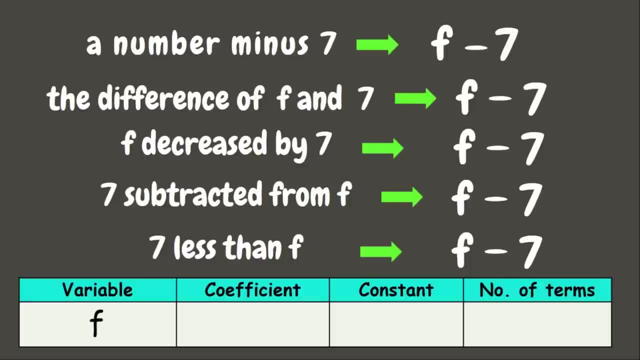 which is very good. It is letter F. And now let us take a look for the coefficient, Since there is no number before our variable here. therefore, the coefficient here is 1.. Next one is the constant. The constant here is negative, 7.. 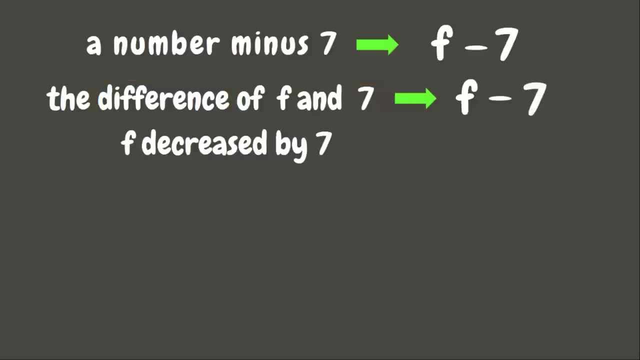 Alright, let us have another example. We have F decreased by 7. So our variable here is F, And we need to decrease this one, which represents subtraction, By 7.. Next example: we have 7 subtracted from F. 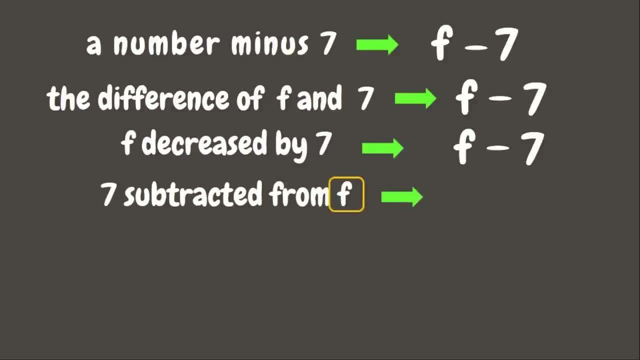 So our variable here is the letter F And we need to subtract 7 from it, So that will be F minus 7.. And lastly, we have 7 less than F And our variable again here is letter F And our keyword is less than. 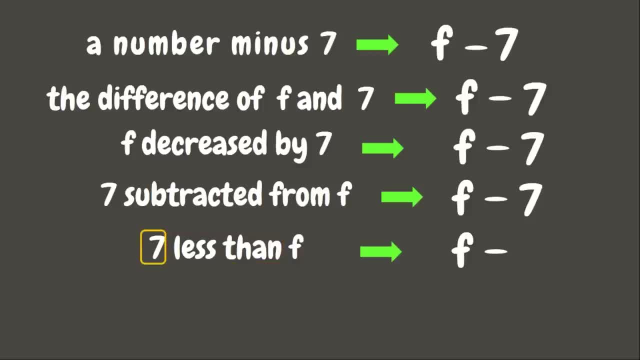 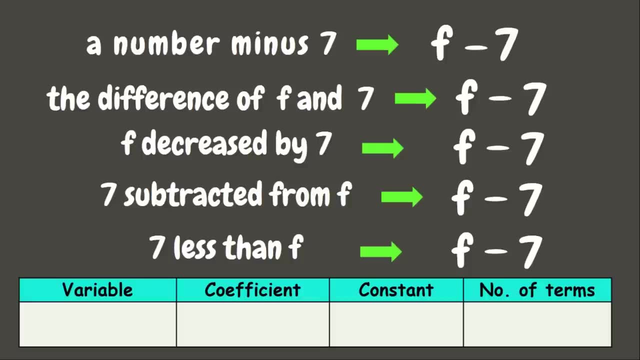 which means subtraction 7.. So that is F minus 7.. Now let us identify the variable. here Again, our variable is the letter, which is Very good. It is letter F. And now let us take a look for the coefficient. 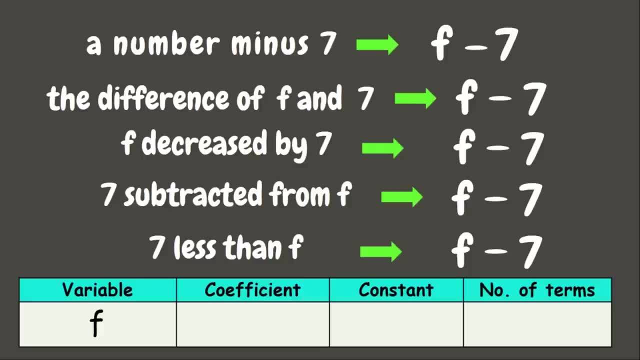 Since there is no number before our variable here. therefore, the coefficient here is 1.. Next one is the constant. The constant here is negative, 7.. Now let us count the number of terms. So we have here minus. that separates the terms. 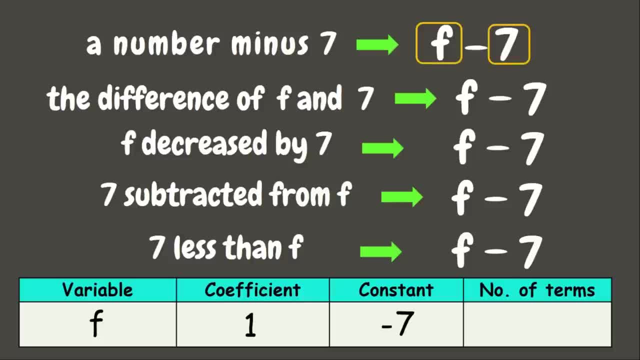 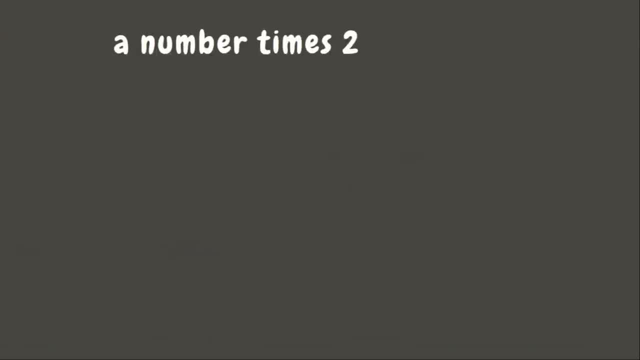 So we have F and 7. So that is 2 terms. Alright, let us go to our next example. This time we have a number times 2. Again, we have here the missing value, which is a number. So now let us represent it by a letter. 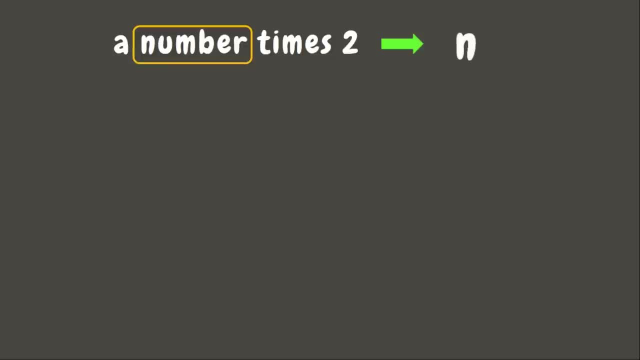 Let us say letter N times, which means multiplication 2. In an algebraic expression, we do not use the multiplication sign as it confuses us into a variable X. Instead of using the multiplication sign, the number, we just simply combine the number and the variable. 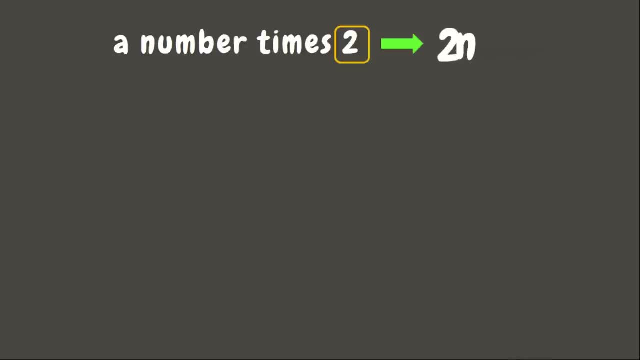 So that would be 2N. Next example: we have twice of N. Here our variable is N and our keyword is the word twice, which means 2 times. So that is 2 times N. Therefore that is 2N. 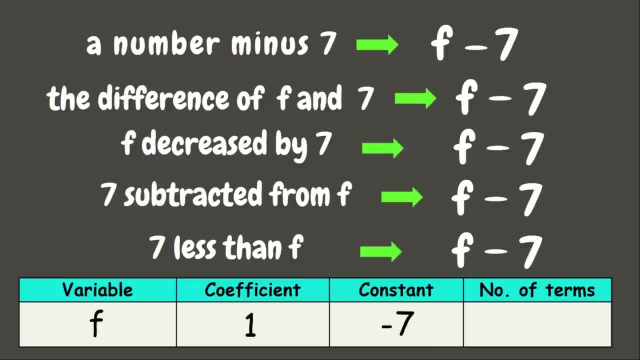 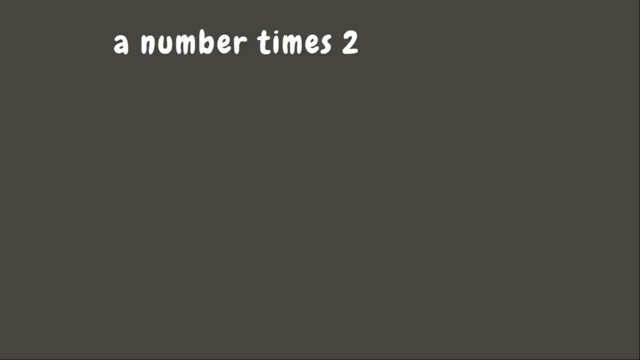 Now let us count the number of terms. So we have here minus. that separates the terms. So we have F and 7. So that is 2 terms. All right, Let us go to our next example. This time we have a number times 2.. 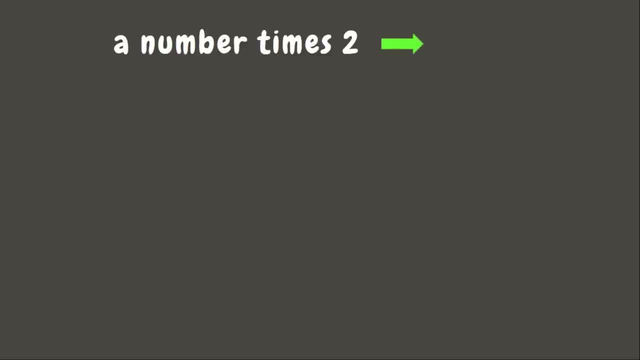 Again, we have here the missing value, which is a number. So now let us represent it by a letter. Let us say letter N times, which means multiplication. 2. In an algebraic expression we do not use the multiplication sign as it confuses us into a variable X. 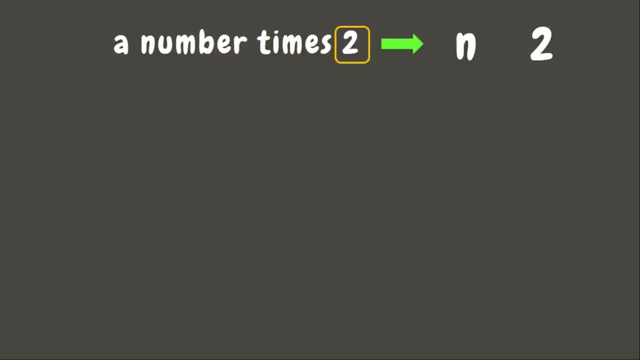 Instead of using the multiplication sign, the number, we just simply combine the number and the variable, So that would be 2N. Next example: we have twice of N. Here our variable is N and our keyword is the word twice, which means 2 times. 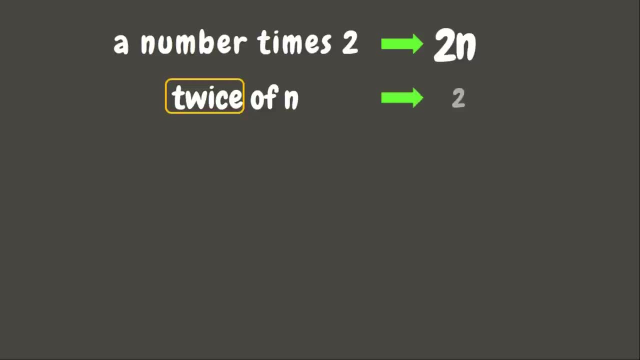 So that is 2 times N. Therefore that is 2N. On to our next example. we have N multiplied by 2.. Here our variable is letter N and our keyword is multiplied by 2. So we need to multiply N by 2.. 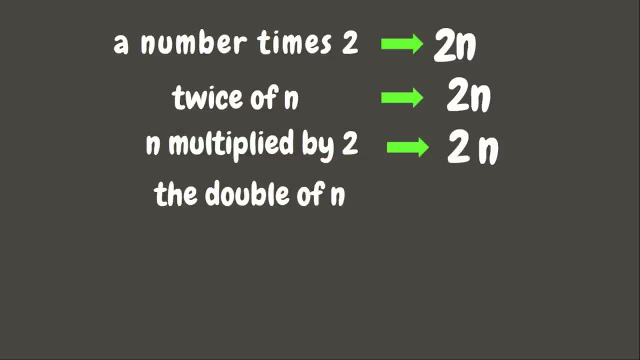 So that would be 2N. Next one: we have the double of N Here. our keyword again is double, which means times 2.. So we need to times 2 the letter N, So that is 2N, Alright. 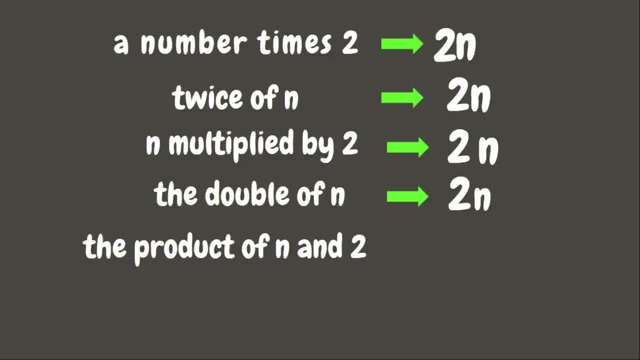 Next one: we have the product of N and 2.. So our variable here is N and our keyword is product, which is the answer for multiplication. This means that we need to multiply N and 2.. So that is 2N. 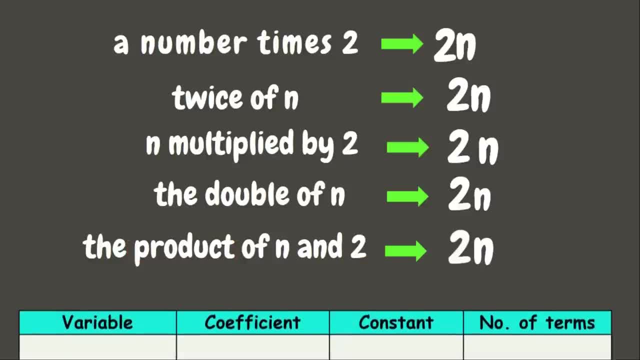 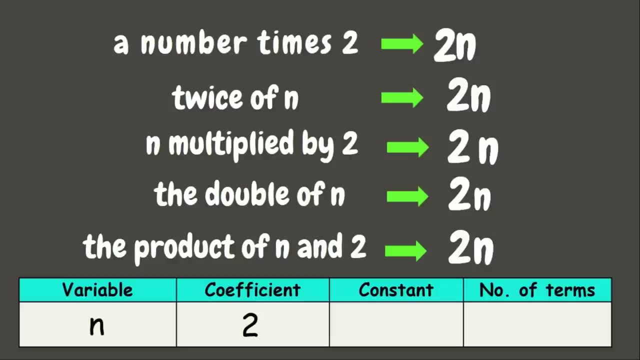 Now let us identify the variable here. The variable here, obviously, is the letter N, while the coefficient is 2, as it is the number before the variable. Next one is the constant. As we can see, we do not have a constant here, While the number of terms 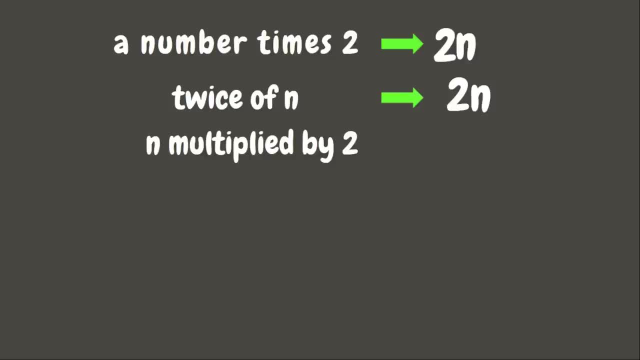 On to our next example. we have N multiplied by 2.. Here our variable is letter N and our keyword is multiplied by 2. So we need to multiply N by 2.. So that would be 2N. Next one: we have the double of N. 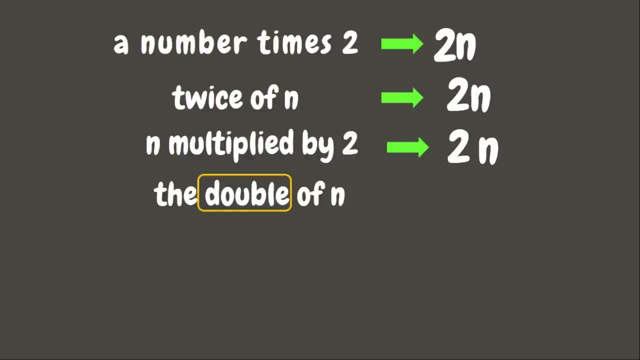 Here our keyword again is double, which means times 2. So we need to times 2 the letter N, So that is 2N. Alright, Next one: we have the product of N and 2.. So our variable here is N. 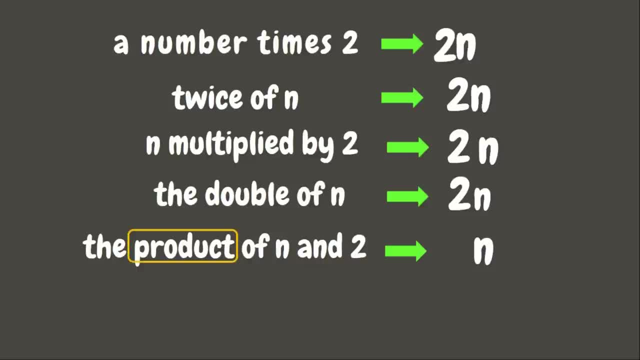 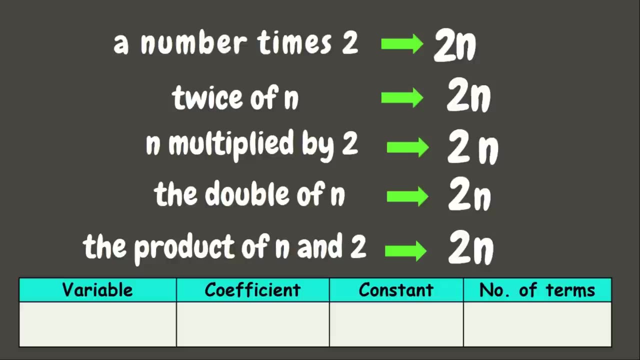 and our keyword is product, which is the answer for multiplication. This means that we need to multiply N and 2.. So that is 2N. Now let us identify the variable here. The variable here obviously is the letter N, while the coefficient is 2. 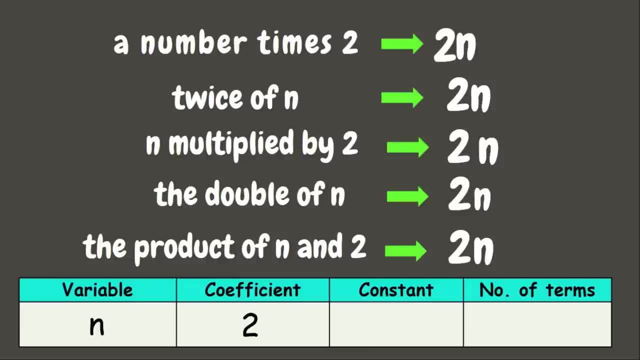 as it is the number before the variable. Next one is the constant. As we can see, we do not have a constant here, While the number of terms, since there is no addition or subtraction that separates the term, we only have one term. 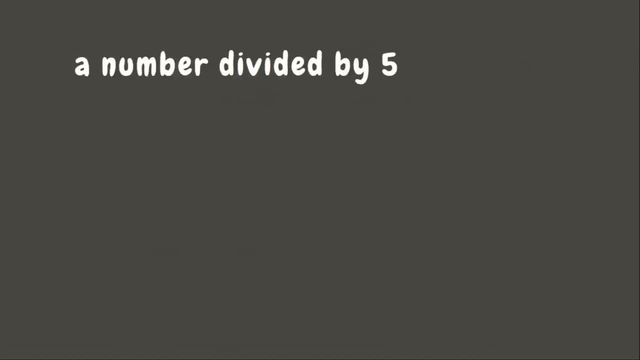 Now let us move on to our next example. Next one: we have a number divided by 5. Again, we have the missing value, which is a number. So let us represent this by a variable N, And we need to divide this by 5.. 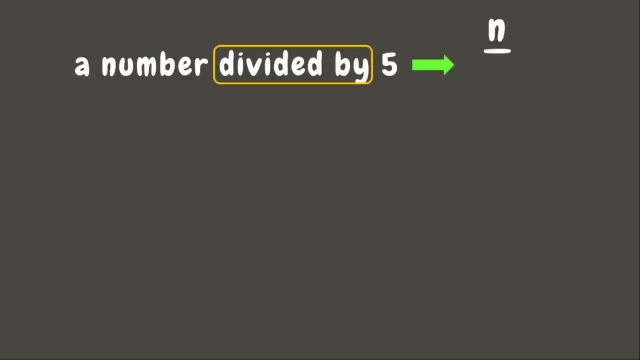 So we can write this as N divided by 5.. Next one: we have the quotient of N and 5.. So again, our keyword here is the quotient, which means division. So it means that we need to divide N and 5.. 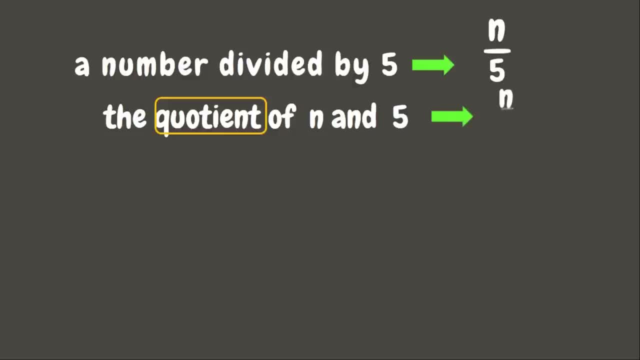 So that is N divided by 5.. Next one: we have one-fifth of N, So it means that we need to multiply one-fifth of N. So that is one-fifth of N, But it can also be written as N over 5.. 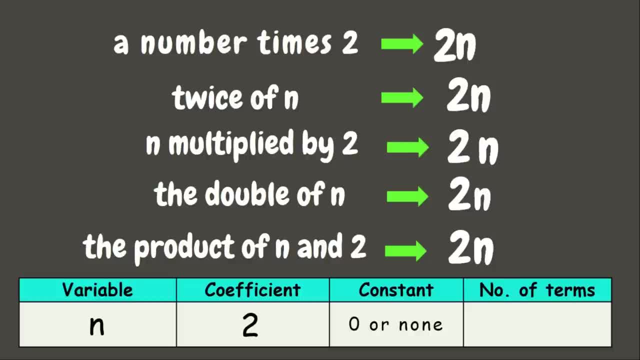 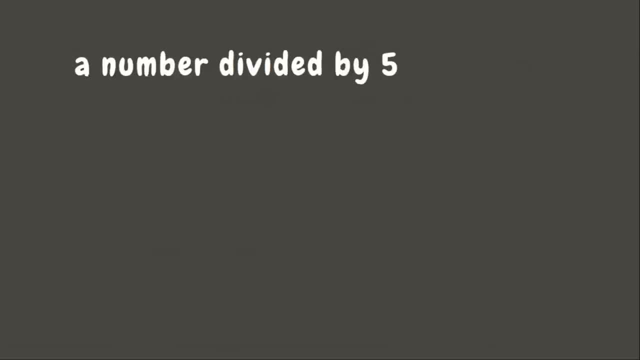 since there is no addition or subtraction that separates the term, we only have one term. Now let us move on to our next example. Next one: we have a number divided by 5. Again, we have the missing value, which is a number. 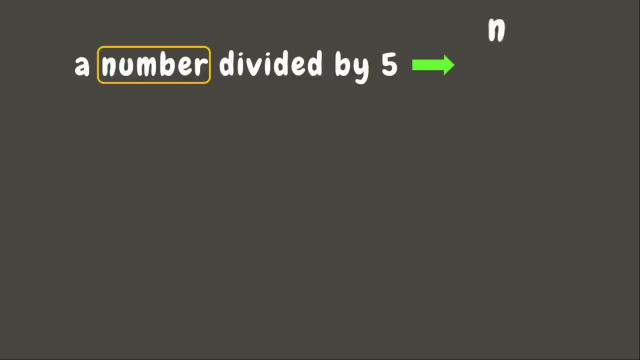 So let us represent this by a variable N, And we need to divide this by 5.. So we can write this as N divided by 5.. Next one: we have the quotient of N and 5.. So again, our keyword here is the quotient. 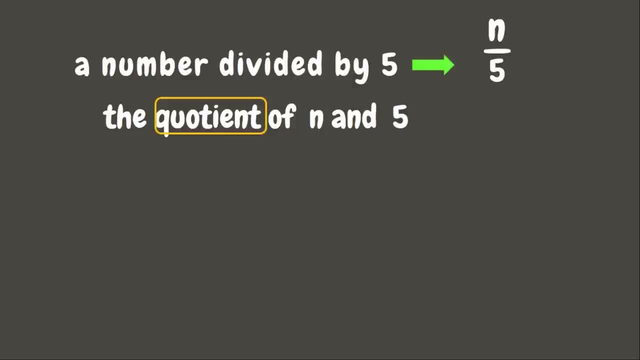 which means division. So it means that we need to divide N and 5.. So that is N divided by 5.. Next one: we have one fifth of N, So it means that we need to multiply one fifth and N. So that is one fifth N. 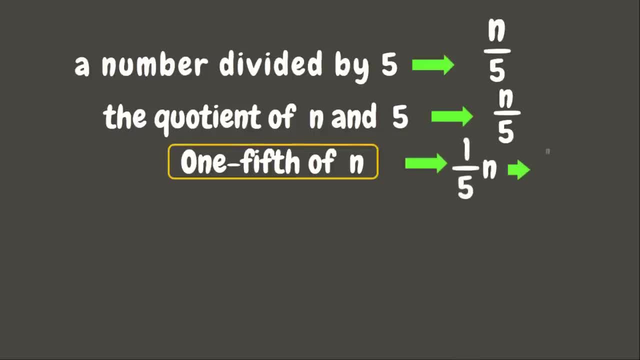 But it can also be written as N over 5.. Okay, next one: we have the ratio of N to 5. Our variable here is N And our clue word here is the ratio of. We all know that we can represent ratio by a fraction. 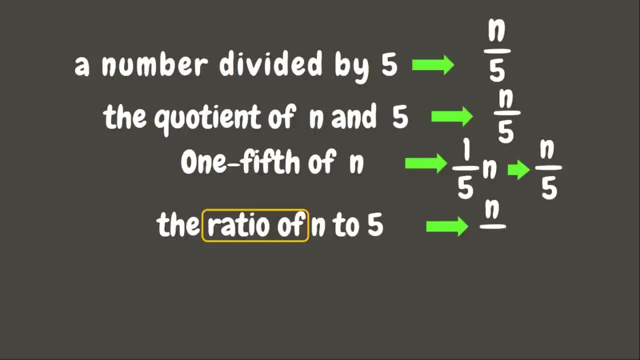 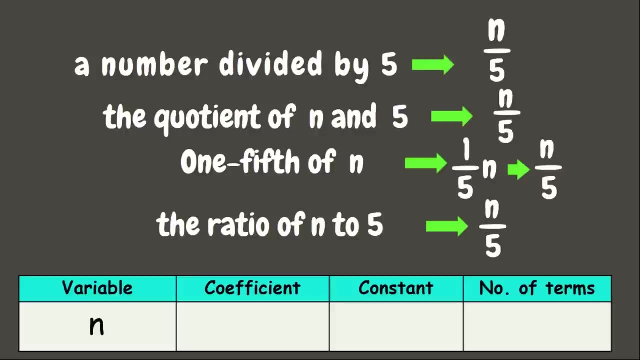 So that would be, N is to 5 or N over 5, which also means N divided by 5.. Now our variable here is the letter N, While the coefficient here is one fifth, As this is the factor or the number being multiplied to the variable N. 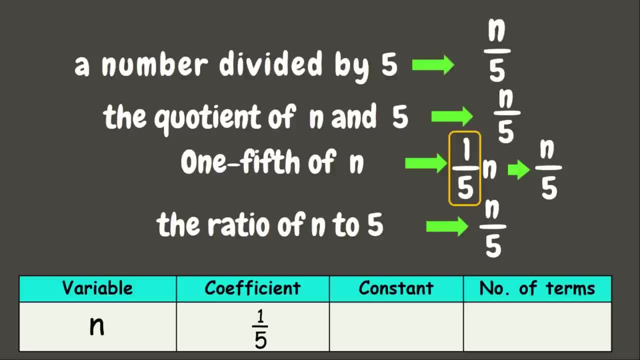 Next one is the constant. Here we cannot see a constant, So that would be 0 or none, While the number of terms, since there's no addition or subtraction that separate the terms, this means that we only have one term: Hooray job. 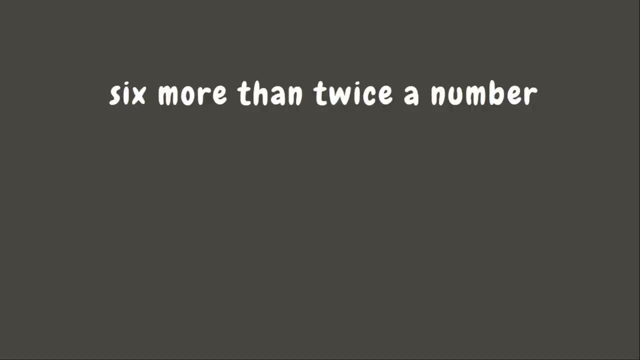 Now that you already know some basics, this time let's try to translate a verbal expression with more than one operations into algebraic expression. Let's have our first example: 6, more than twice a number. So again we need to take a look for some clue words. 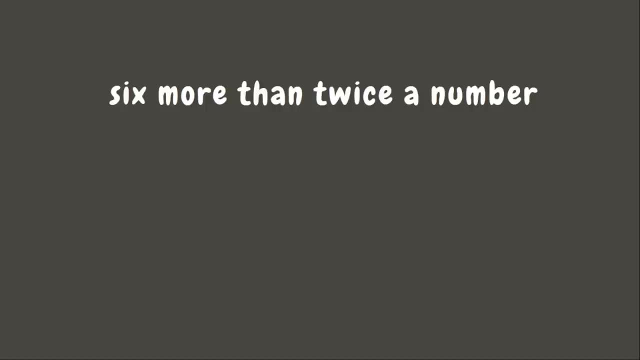 in order for us to translate this one. So our clue word here, as we can see, we have twice a number And we all know that that means 2 times a number or a variable. So we can say that is 2a. 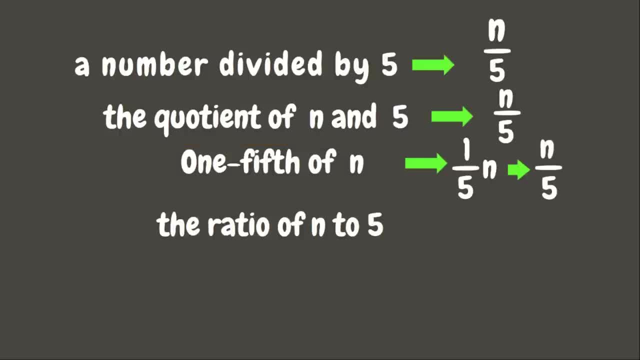 Next one: we have the ratio of N to 5.. Our variable here is N And our clue word here is the ratio of. We all know that we can represent ratio by a fraction, So that would be N is to 5 or N over 5.. 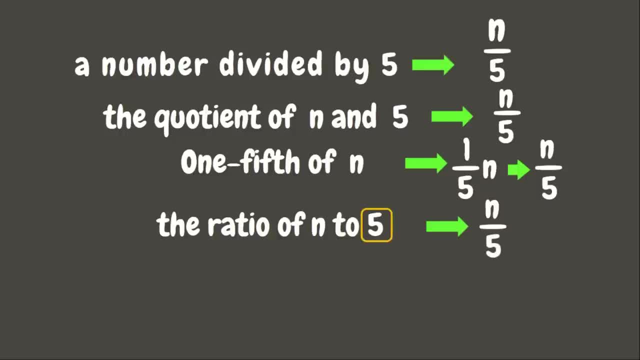 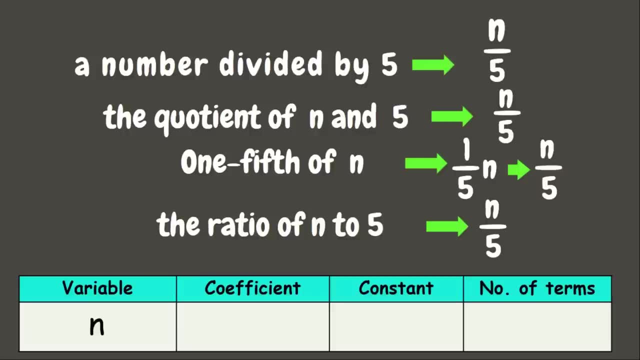 Which also means N divided by 5.. Now our variable here is the letter N, While the coefficient here is one-fifth, As this is the factor or the number being multiplied to the variable N. Next one is the constant. Here we cannot see a constant. 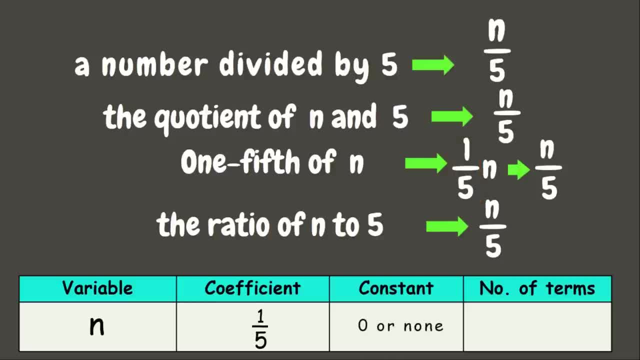 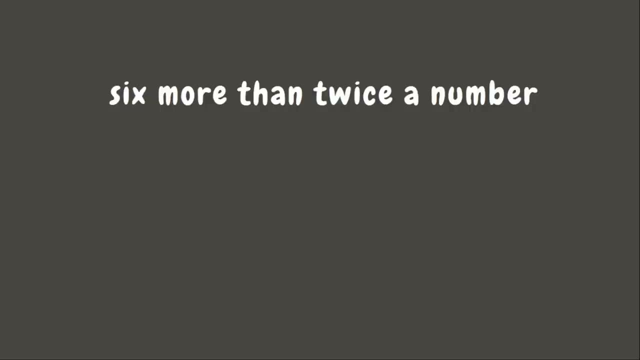 So that would be 0 or none. While the number of terms? there is no addition or subtraction that separates the terms. This means that we only have one term: Hooray job. Now that you already know some basics, This time let's try to translate. 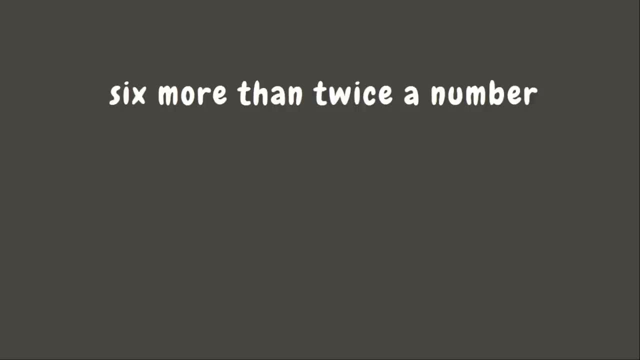 a verbal expression with more than one operations into algebraic expression. Let's have our first example: 6, more than twice a number. So again we need to take a look for some clues in order for us to translate. So our clue word here: 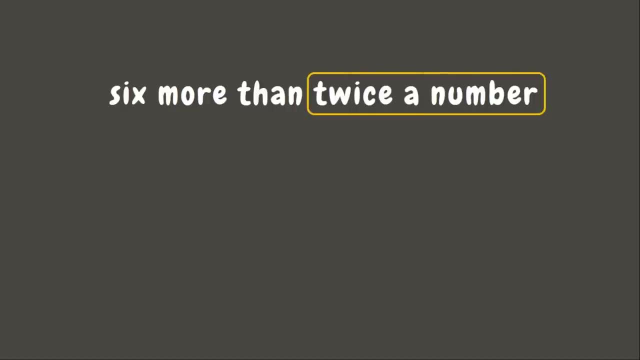 as we can see, we have twice a number And we all know that that means 2 times a number or a variable. So we can say that is 2a And next one we have 6 more than, And that is plus 6.. 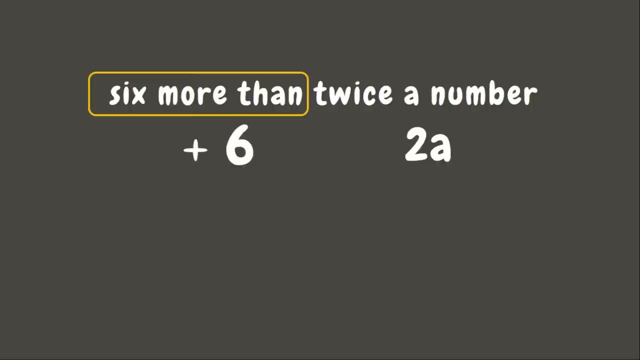 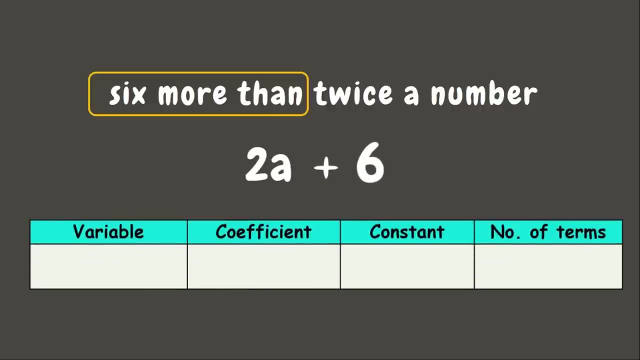 So therefore our expression here is 2a plus 6.. Wonderful, Now let's identify the variable. here is a Good job. Well, the coefficient here is 2.. Next one: the constant is 6.. And we have here 2 terms. 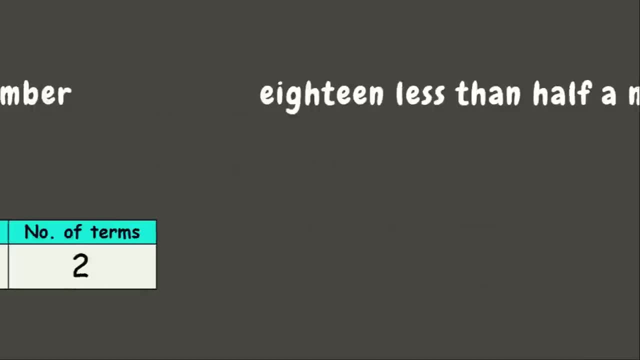 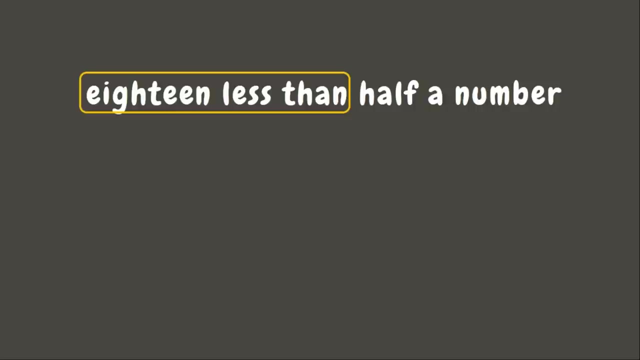 which are 2a and 6.. Let's have another example. This time we have 18 less than half a number. Now let's take a look for some keywords. We have here 18 less than, And we all know that less than means subtract. 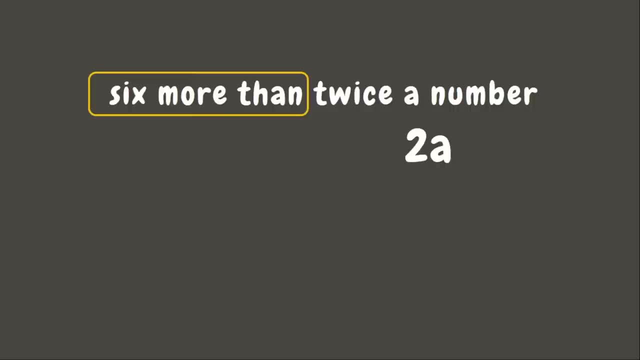 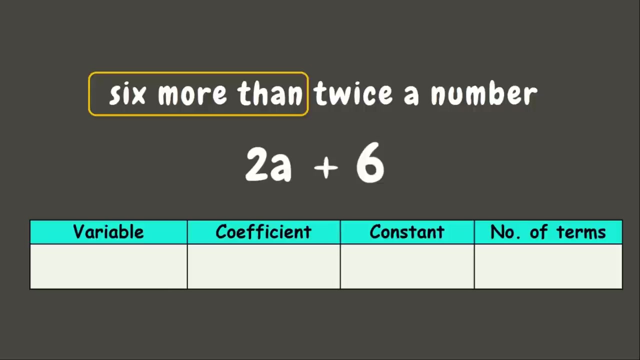 And next one: we have 6 more than, And that is plus 6.. So therefore, our expression here is 2a plus 6.. Wonderful. Now let's identify the variable. here is a Good job. Well, the coefficient here is 2.. 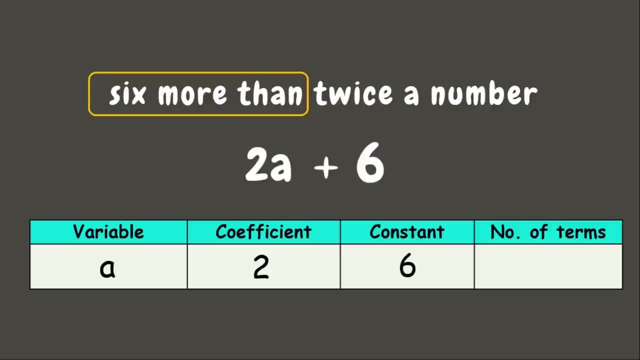 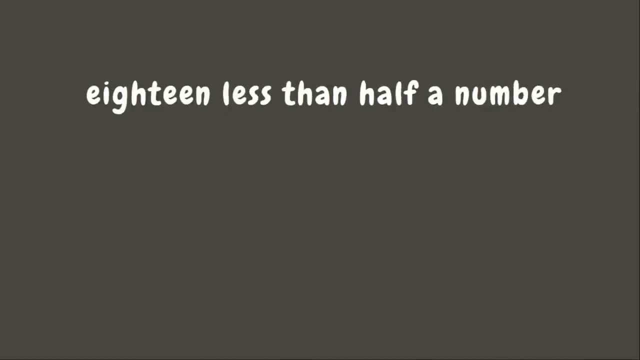 Next one: the constant is 6. And we have here 2 terms, which are 2a and 6.. Let's have another example. This time we have 18, less than half a number. Now let's take a look for some clue words. 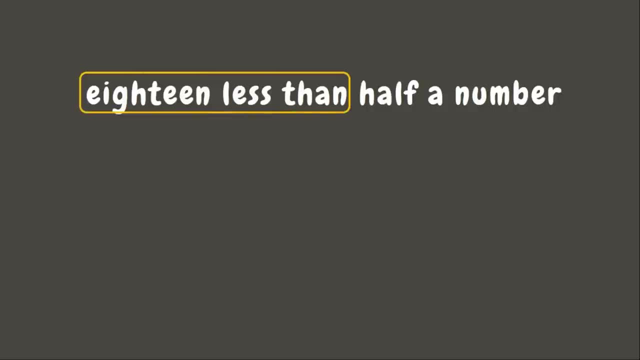 We have here 18 less than, And we all know that less than means subtract, So that is minus 8.. Next one: we have half a number, And that means 1 half times a number or a variable, So that would be 1 half y. 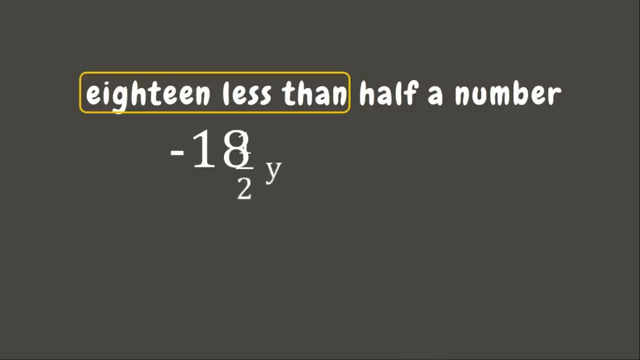 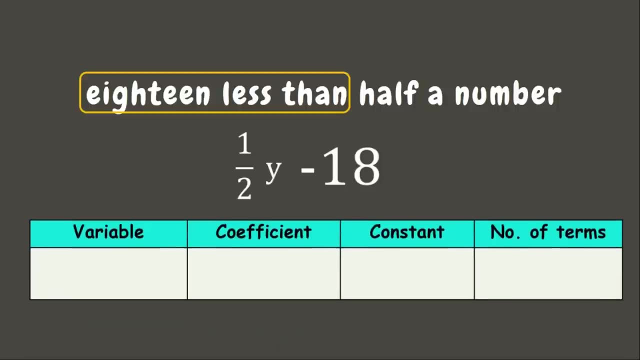 Now, if we combine them together, we have 1 half y minus 8. So that is 18 less than half a number. So here our variable is y. Well, the coefficient here is 1 half. Well, the constant is negative, 18 or minus 18.. 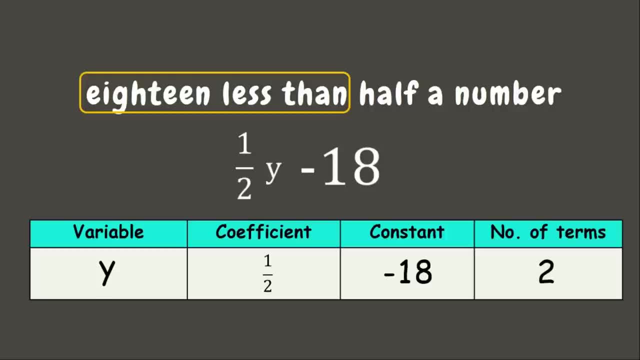 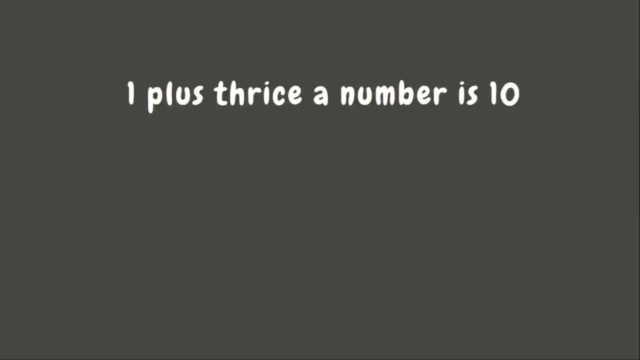 And the number of terms here are 2.. That is 1 half y and 18.. Now let's have another example. We have 1 plus twice a number is 10.. So our first clue word here is twice a number, And that means 3 times a variable. 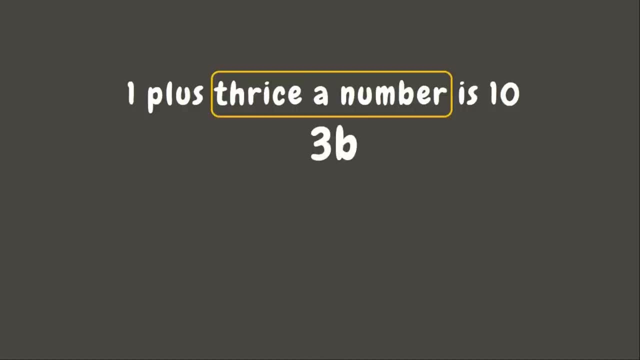 So we can say it is 3b. Next one, we have 1 plus, And that means plus 1.. If we combine that together, we have 3b plus 1.. And we still have more to translate. Here we have the word is 10,. 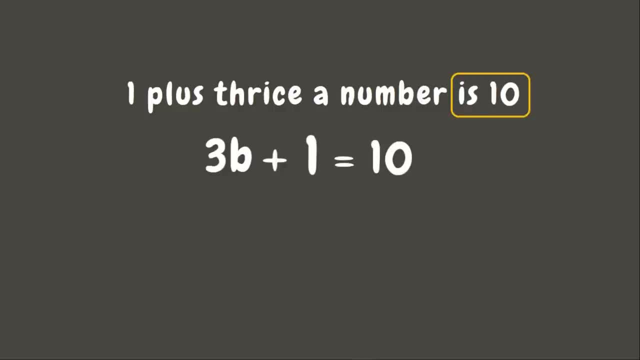 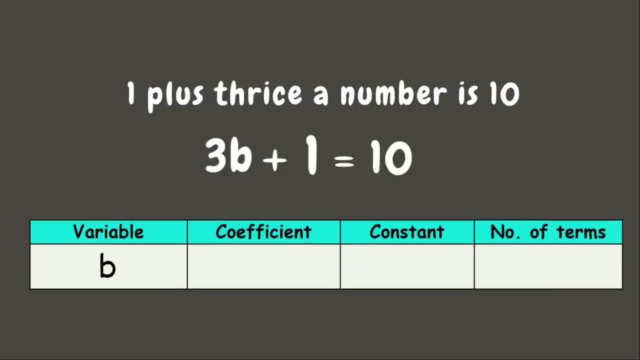 which means that equals 10.. So that is 3b plus 1 equals 10.. So here we have the variable b. Well, the coefficient here is 3.. The constants are 1 and 10. And the number of terms here are 3,. 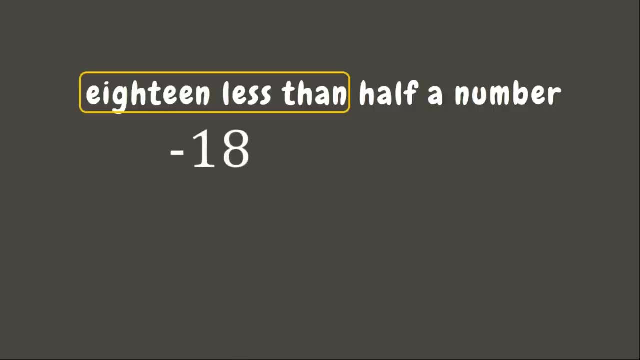 So that is minus 8.. Next one: we have half a number, And that means 1 half times a number or a variable, So that would be 1 half y. Now if we combine them together, we have 1 half y minus 8.. 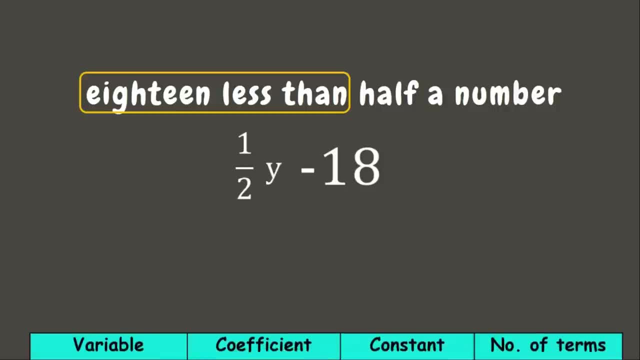 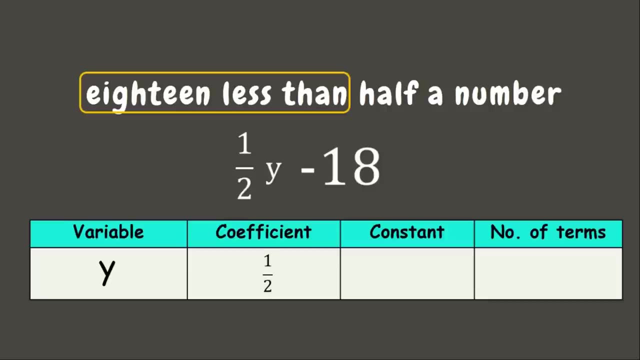 So that is 18 less than half a number. So here our variable is y. Well, the coefficient here is 1, half, While the constant is negative, 18 or minus 18.. And the number of terms here are 2.. 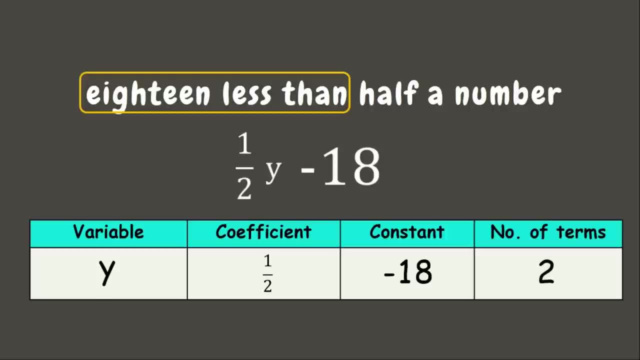 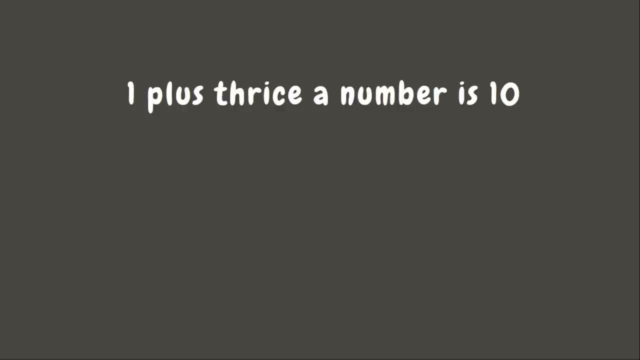 That is 1 half y and 18.. Now let's have another example. We have: 1 plus twice a number is 10.. So our first clue word here is twice a number, And that means 3 times a variable. So we can say it is 3b. 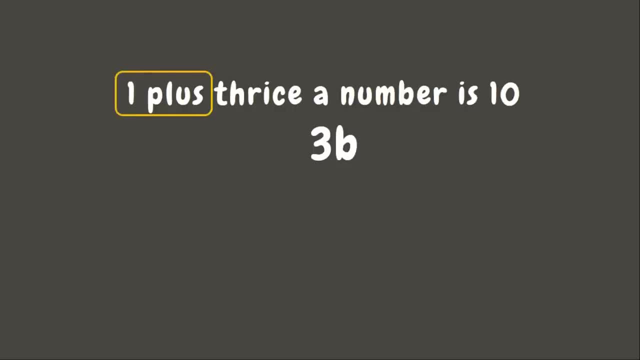 Next one: we have 1 plus, And that means plus 1. If we combine that together, we have 3b plus 1. And we still have more to translate. Here we have the word is 10. Which means that equals 10.. 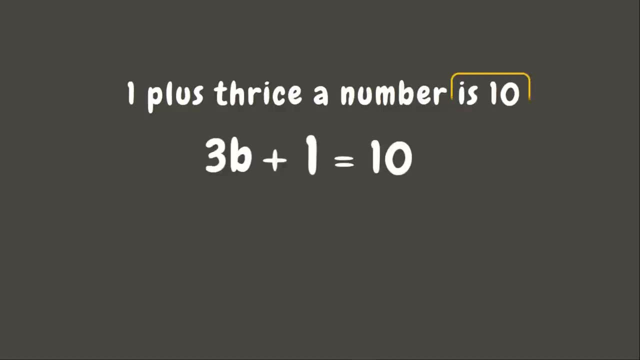 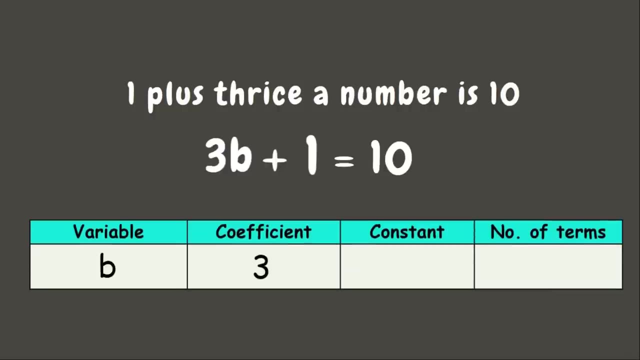 So that is, 3b plus 1 equals 10.. So here we have the variable b, While the coefficient here is 3, the constants are 1 and 10. And the number of terms here are 3.. Which are 3b, 1 and 10.. 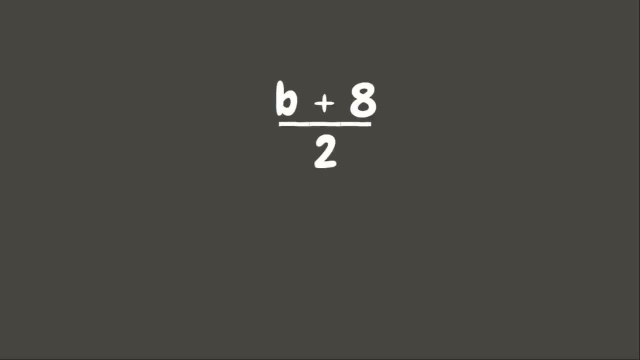 This time let us translate an expression into a verbal or word, sentences or phrases. Here we have b plus 8 divided by 2. So first we have b plus 8. We can write this one as sum of b and 8.. 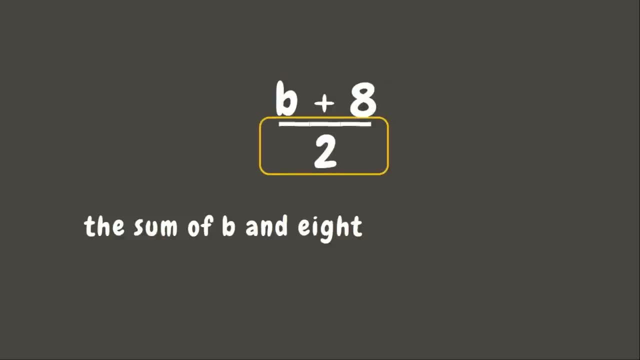 And next we have divided by 2. So that would be divided by 2.. Now we have the sum of b and 8 divided by 2. Wonderful. Let us have another example Here we have 3n plus 25 equals 31..